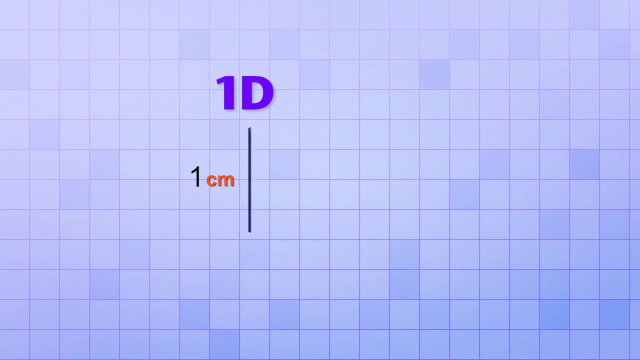 And in the Math Antics video about area we saw that if we move or extend this one-dimensional line in a direction perpendicular to it by a distance of one centimeter, it forms a two-dimensional object called a volume. The two-dimensional objects are measured by the two-dimensional quantity that we call area. 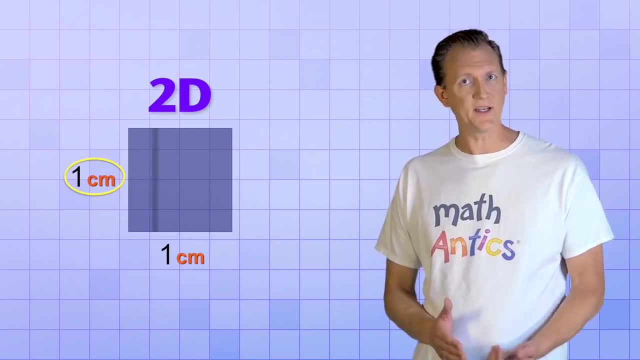 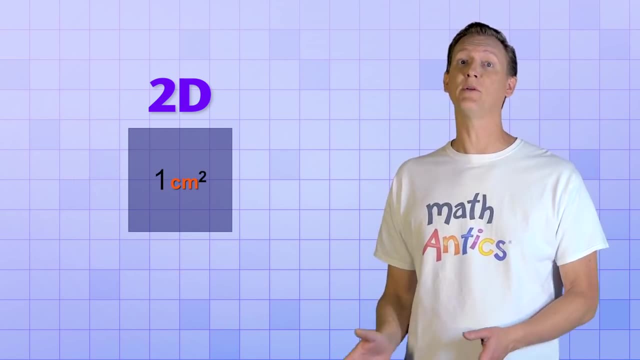 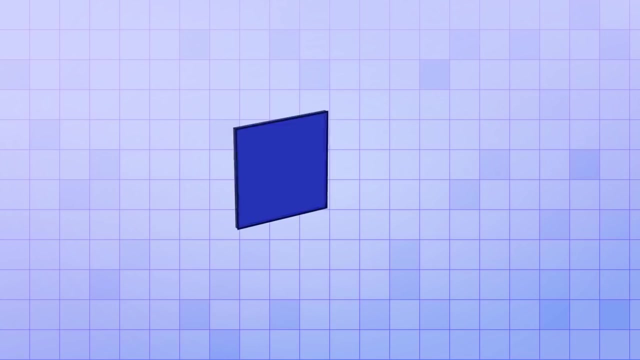 Because the original line was one centimeter long and we extended it a distance of one centimeter. the amount of area that this square occupies is one square centimeter, which is a common unit for measuring area. OK, now imagine that we take that two-dimensional square and move or extend it. 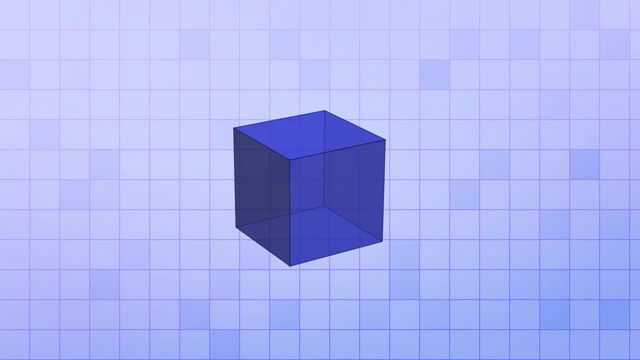 in a direction perpendicular to its surface by a distance of one centimeter, It forms a three-dimensional object that's called a cube. It forms a three-dimensional object that's called a cube, And to measure a three-dimensional object like this, we use a three-dimensional quantity called volume. 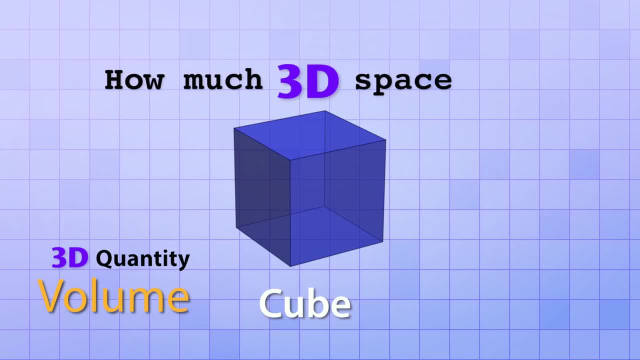 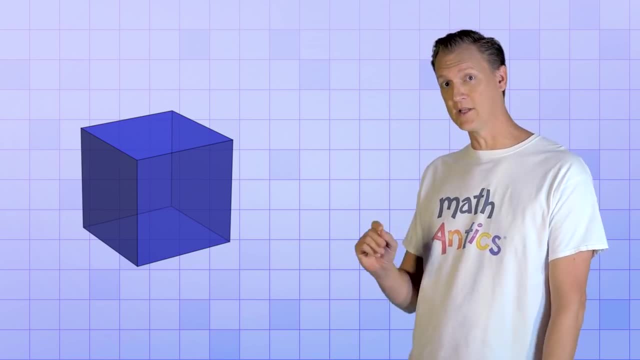 Volume tells us how much three-dimensional space, or 3D space, an object occupies. Alright, but how much volume does this cube have? Well, since it was made by extending one square centimeter, a distance of one centimeter in the third dimension, 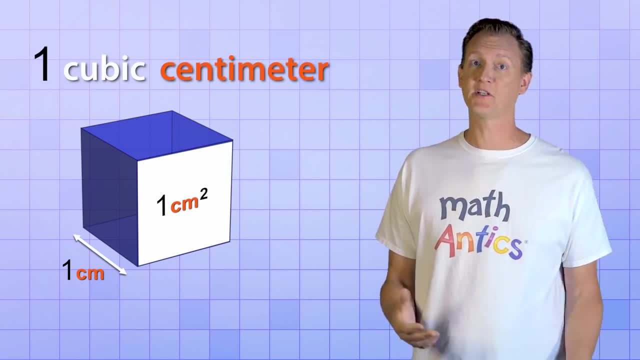 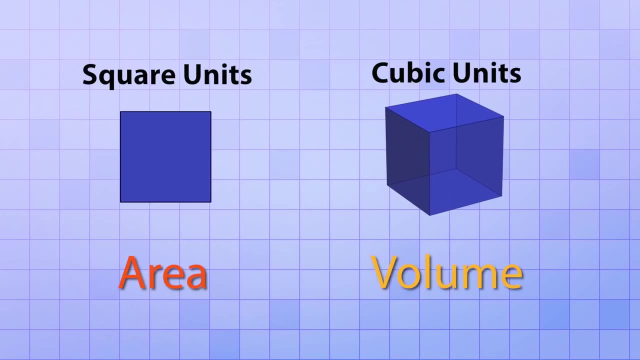 we say that its volume is exactly one cubic centimeter, which is a common unit for measuring volume. So square units are used to measure area and cubic units are used to measure volume, Since square units are made by multiplying two one-dimensional units together, like centimeter times centimeter. 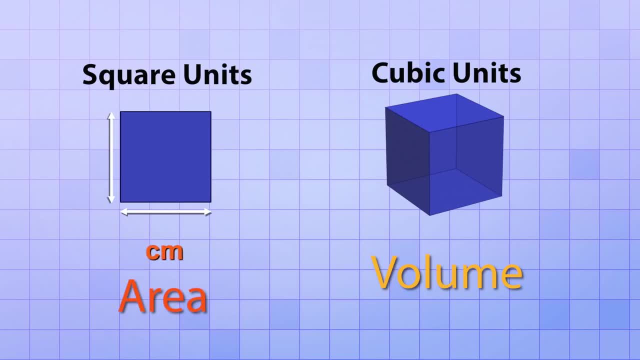 we can abbreviate them using the exponent notation centimeters to the second power or centimeters squared. And since cubic units are made by multiplying three one-dimensional units together, like centimeter times centimeter times centimeter, we can abbreviate them using exponent notation. 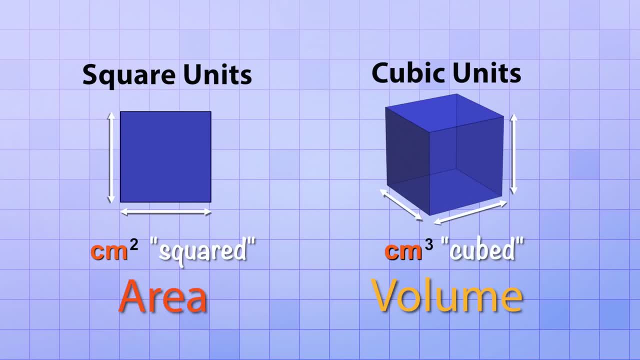 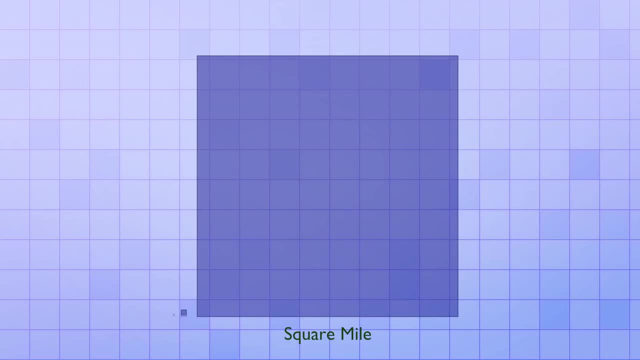 centimeters to the third power, or centimeters cubed. And just like there were different sizes of square units like square inches, square meters or square miles, there's also different sized cubic units like cubic inches, cubic meters or cubic miles. 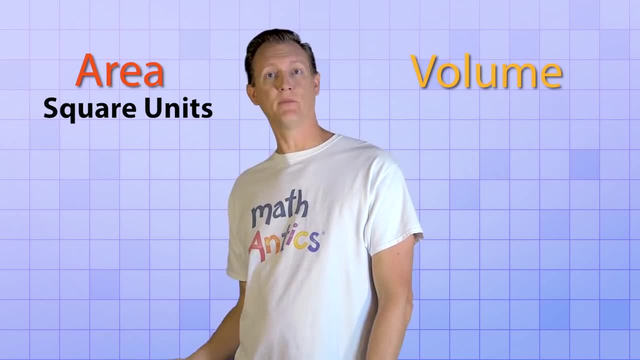 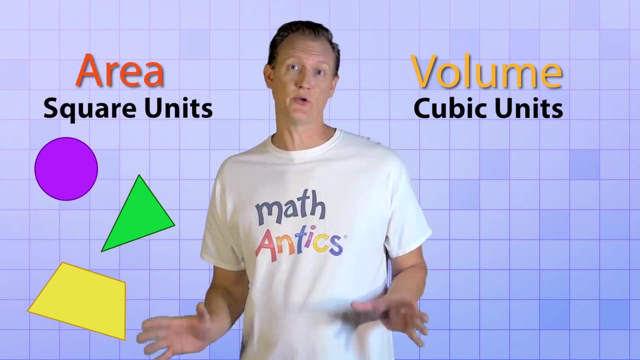 See how area and square units are related to volume and cubic units. And there's another similarity too. Do you remember how you can use square units to measure the area of ANY 2D shape, not just squares? Well, you can use cubic units to measure the volume of ANY 3D shape, not just squares. 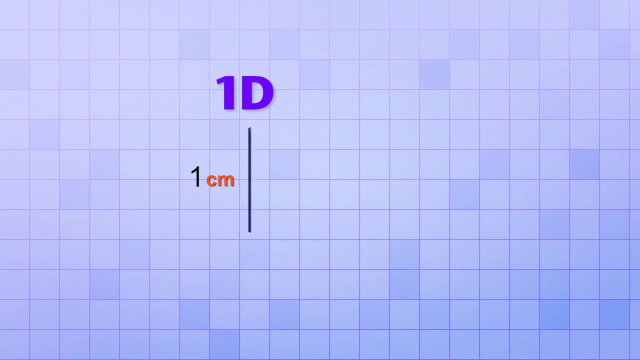 And in the Math Antics video about area we saw that if we move or extend this one-dimensional line in a direction perpendicular to it by a distance of one centimeter, it forms a two-dimensional object called a volume. The two-dimensional objects are measured by the two-dimensional quantity that we call area. 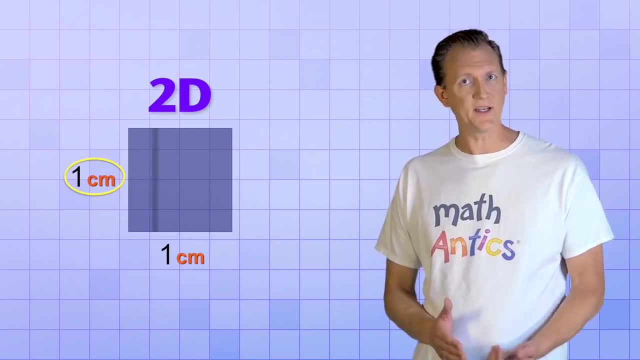 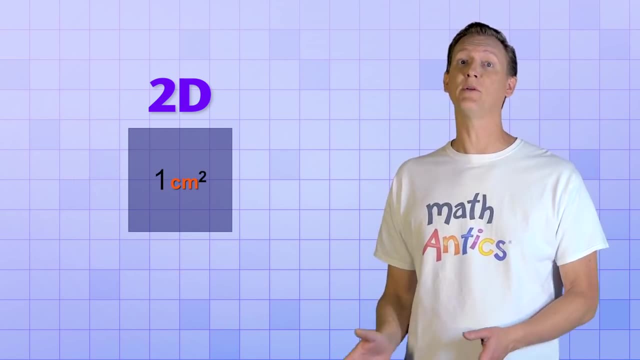 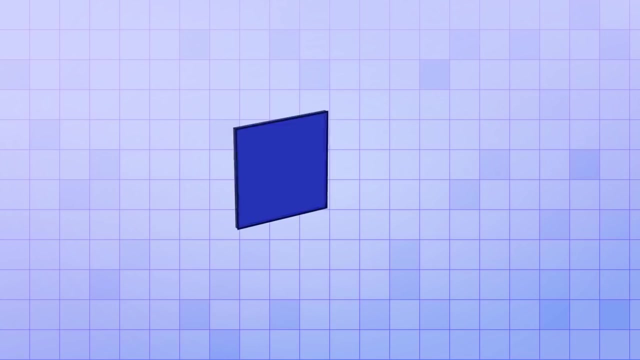 Because the original line was one centimeter long and we extended it a distance of one centimeter. the amount of area that this square occupies is one square centimeter, which is a common unit for measuring area. OK, now imagine that we take that two-dimensional square and move or extend it. 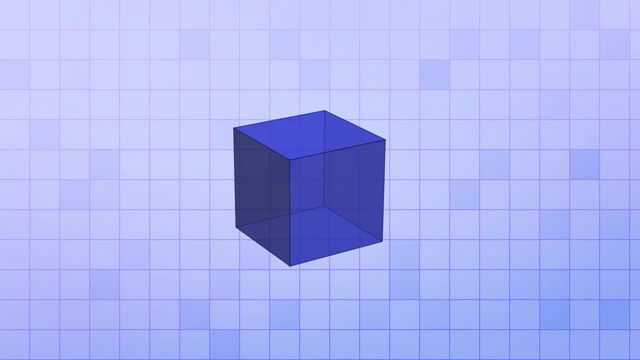 in a direction perpendicular to its surface by a distance of one centimeter, It forms a three-dimensional object that's called a cube. It forms a three-dimensional object that's called a cube, And to measure a three-dimensional object like this, we use a three-dimensional quantity called volume. 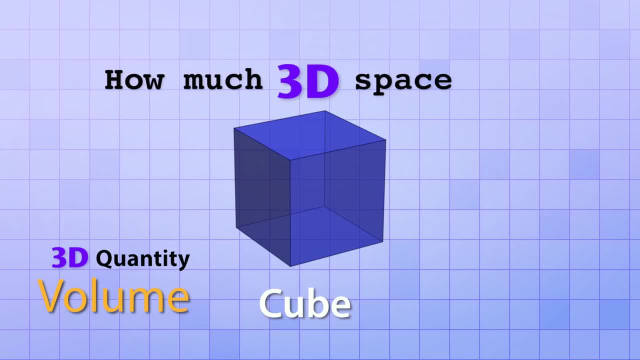 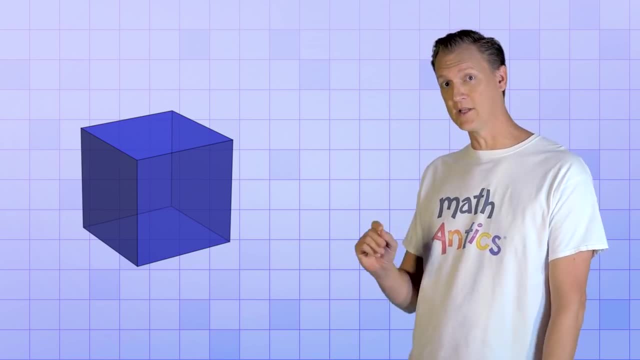 Volume tells us how much three-dimensional space, or 3D space, an object occupies. Alright, but how much volume does this cube have? Well, since it was made by extending one square centimeter, a distance of one centimeter in the third dimension, 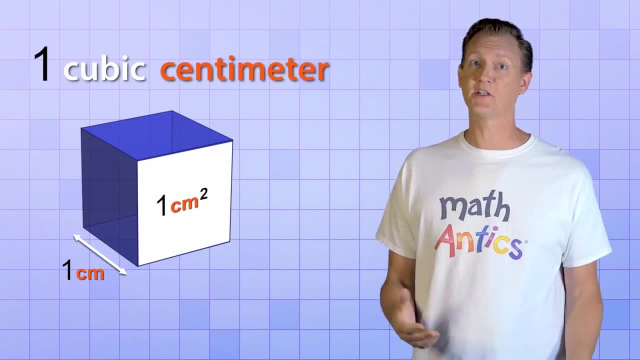 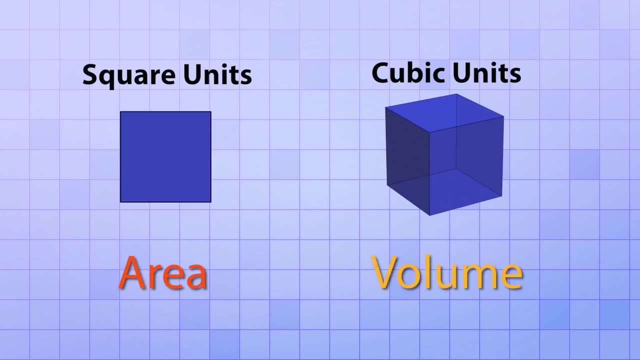 we say that its volume is exactly one cubic centimeter, which is a common unit for measuring volume. So square units are used to measure area and cubic units are used to measure volume, Since square units are made by multiplying two one-dimensional units together, like centimeter times centimeter. 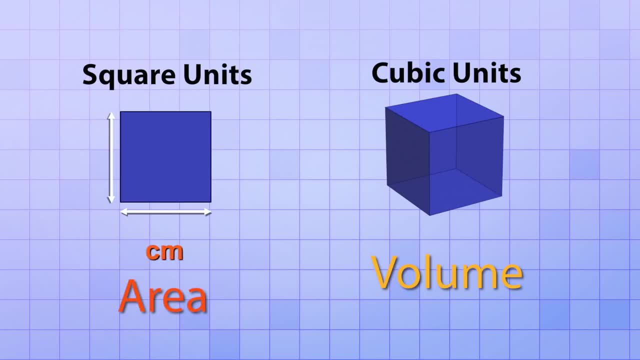 we can abbreviate them using the exponent notation centimeters to the second power or centimeters squared. And since cubic units are made by multiplying three one-dimensional units together, like centimeter times centimeter times centimeter, we can abbreviate them using exponent notation. 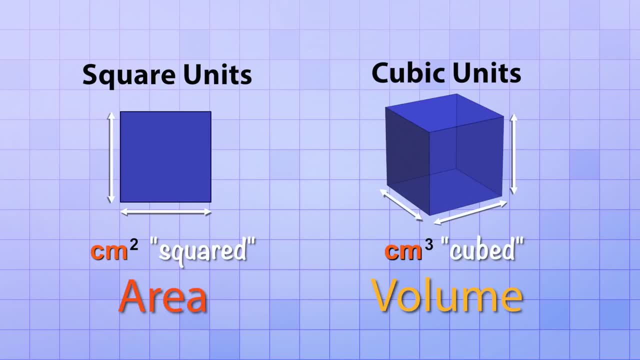 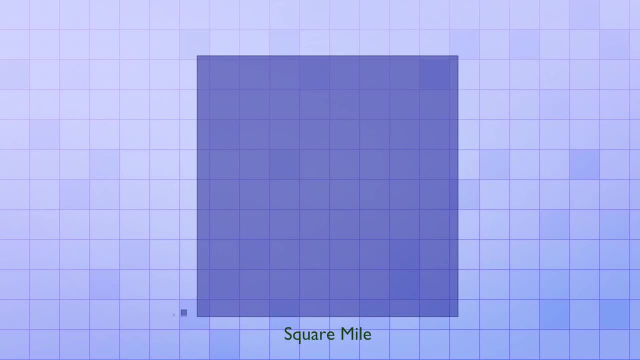 centimeters to the third power, or centimeters cubed. And just like there were different sizes of square units like square inches, square meters or square miles, there's also different sized cubic units like cubic inches, cubic meters or cubic miles. 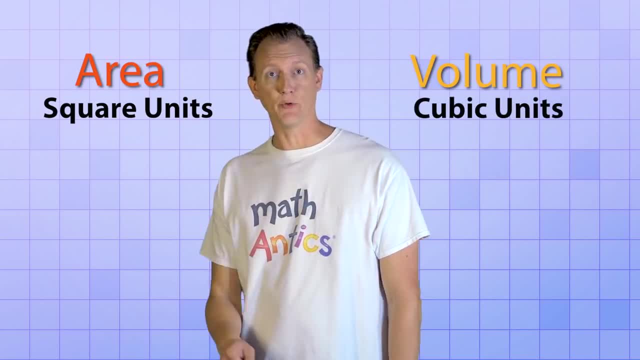 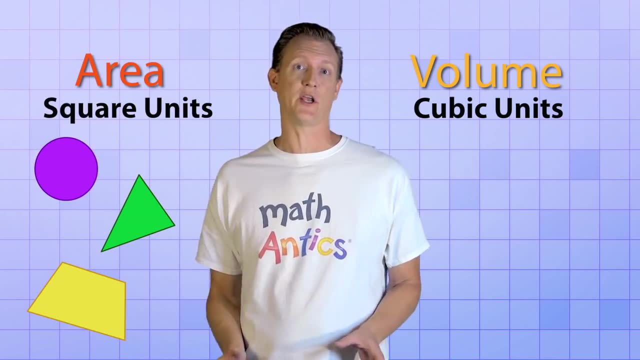 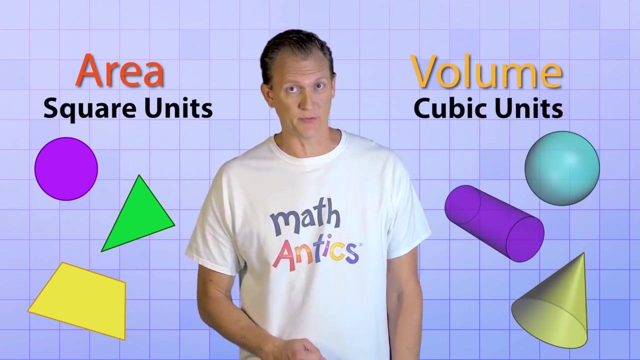 See how area and square units are related to volume and cubic units. And there's another similarity too. Do you remember how you can use square units to measure the area of ANY 2D shape, not just squares? Well, you can use cubic units to measure the volume of ANY 3D shape, not just cubes. 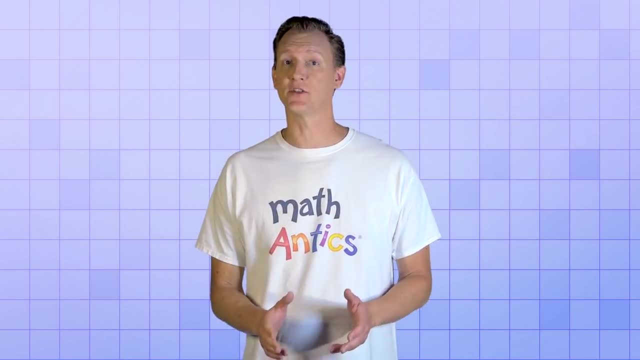 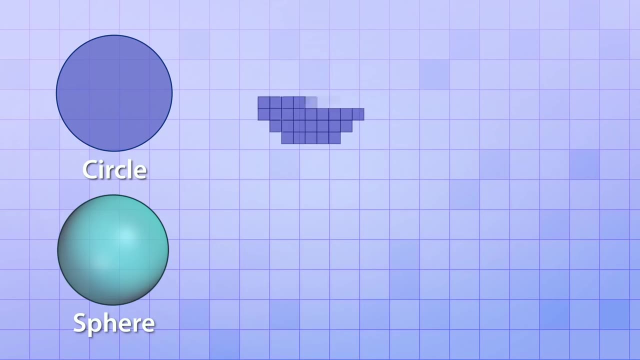 To see how that works, take a look at this 2D circle and this 3D object called a sphere, which is like a ball. Just like you can use a bunch of small squares to approximate the area of the circle, you can use a bunch of small cubes to approximate the volume of the sphere. 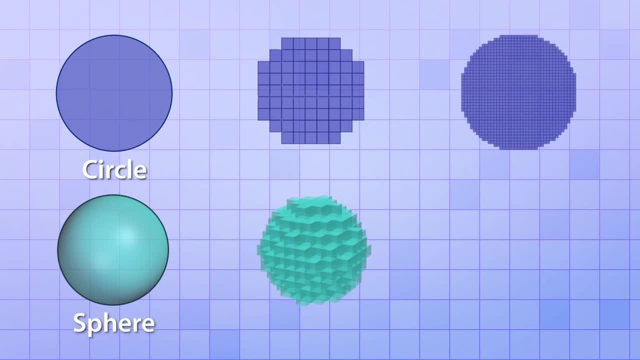 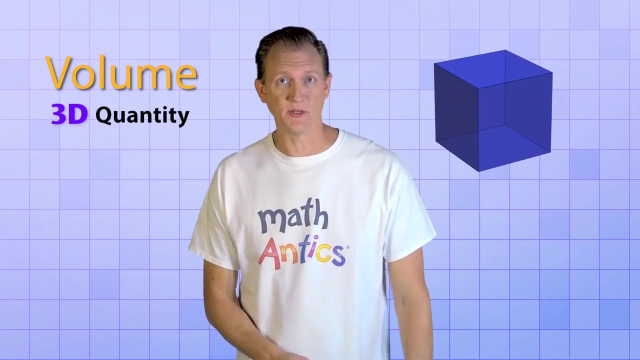 And here's the really cool part: The smaller the squares you use, the closer their combined area will match the area of the circle, And the smaller the cubes you use, the closer their combined volume will match the volume of the sphere. OK, so volume is a 3D quantity for measuring 3D objects. 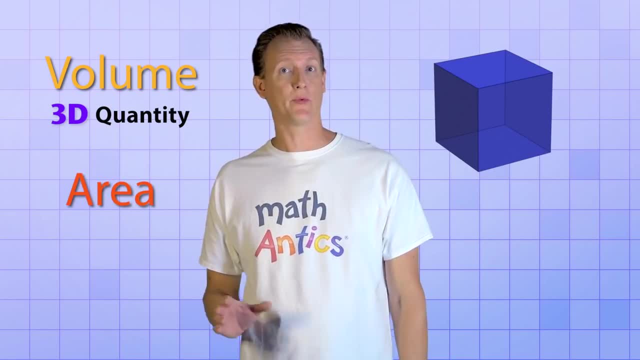 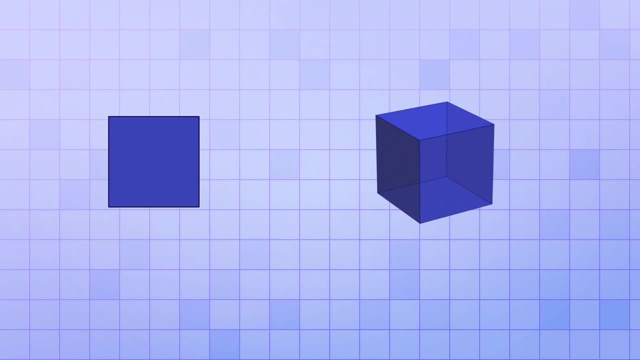 But since we've also talked a lot about area in this video, I want to point out that 3D objects also have a type of area that you don't want to confuse with volume. You might remember from our previous videos that 2D shapes have both a 2D quantity called area and a 1D quantity called perimeter. 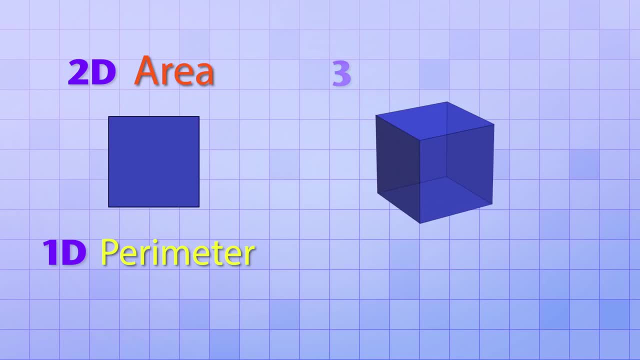 Well, in a similar way, 3D objects have both a 3D quantity called volume and a 2D quantity called surface area. Surface area is a lot like it sounds. It's the area of the object's outer surface or shell. 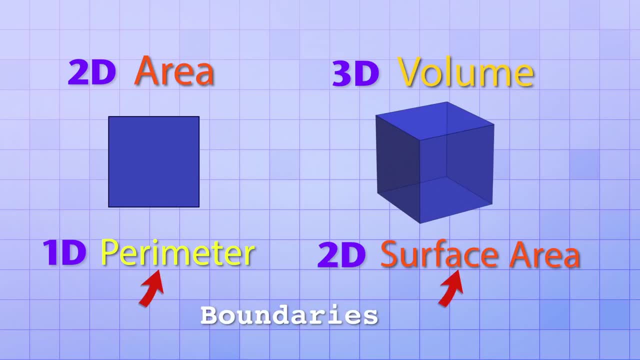 Perimeter and surface area are both outer boundaries of geometric shapes. Perimeter is the one-dimensional outer boundary of a two-dimensional shape And surface area is the two-dimensional outer boundary of a three-dimensional shape. And to help you see the difference between surface area and volume, 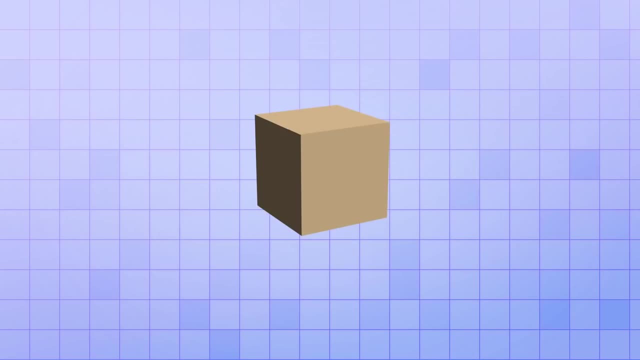 imagine that you have a perfectly thin box filled with ice. If you unfold the box, you can see the 2D area that surrounds it. Well, the volume itself is the amount of 3D space occupied by the ice inside the box. 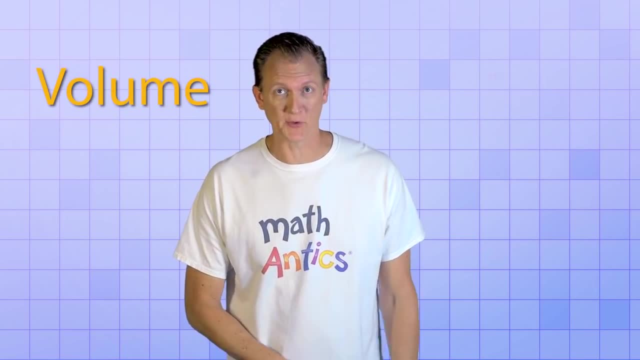 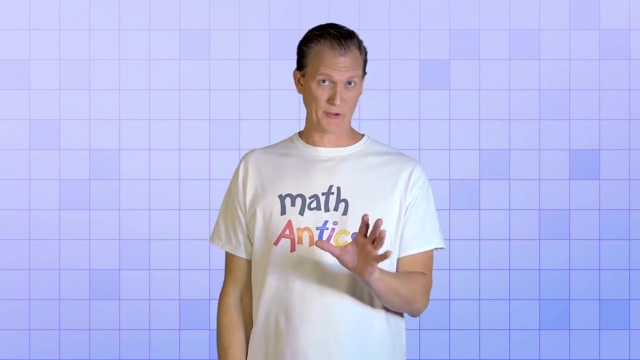 Alright. so now that you understand what volume is and you won't confuse it with surface area, we're going to spend the rest of the video learning how to calculate the volumes of some basic geometric shapes. But before we do that, I want to quickly mention something important about terminology. 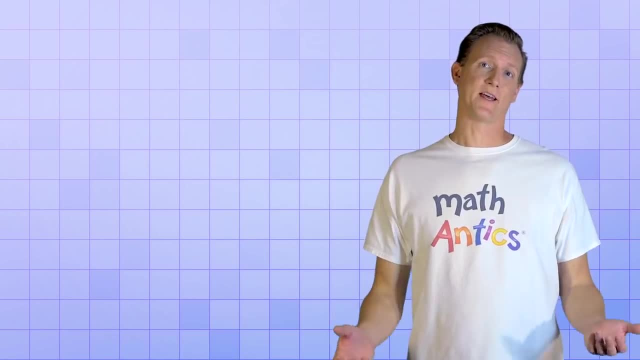 or the words we use to describe things in math. Most of the time, people agree on what to call things in math, but not always, And that's especially true when it comes to the words that we use to describe things in math. Most of the time, people agree on what to call things in math, but not always. 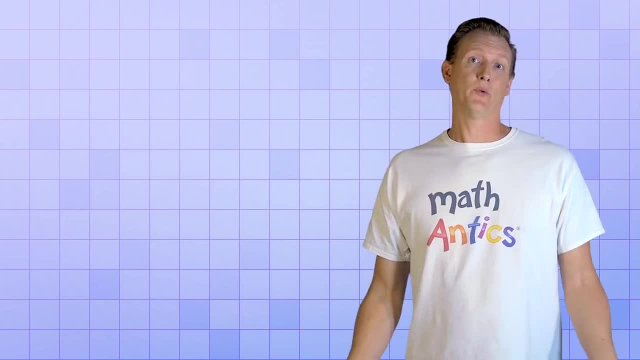 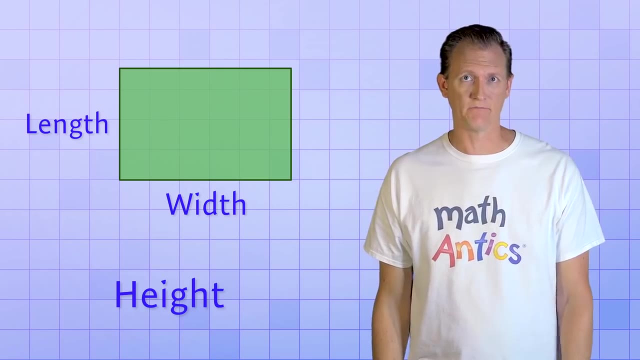 And that's especially true when it comes to the words that we use to describe things in math. Take the words length, width and height, for example. If I have a rectangle, I could name its two dimensions, length and width, like we did in the area video. 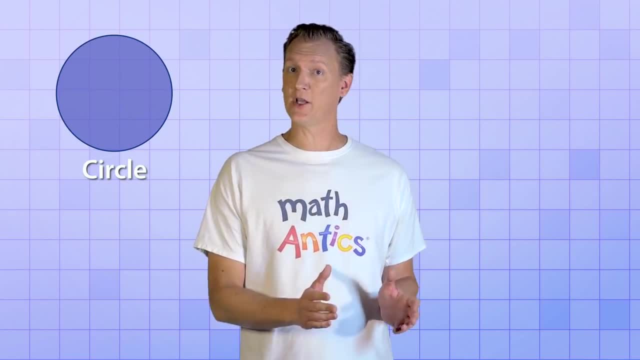 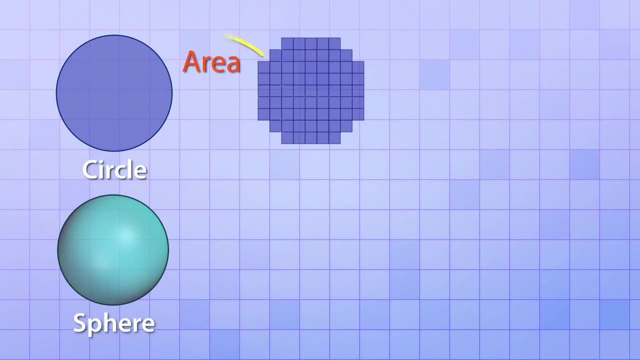 To see how that works, take a look at this 2D circle and this 3D object called a sphere, which is like a ball. Just like you can use a bunch of small squares to approximate the area of the circle, you can use a bunch of small cubes to approximate the volume of the sphere. 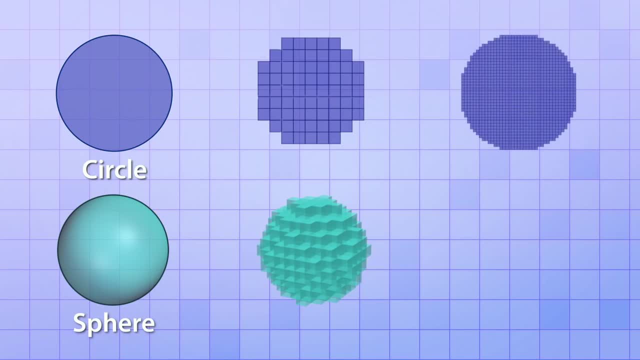 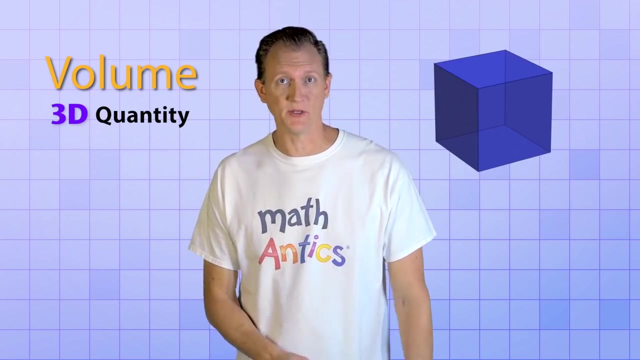 And here's the really cool part: The smaller the squares you use, the closer their combined area will match the area of the circle, And the smaller the cubes you use, the closer their combined volume will match the volume of the sphere. OK, so volume is a 3D quantity for measuring 3D objects. 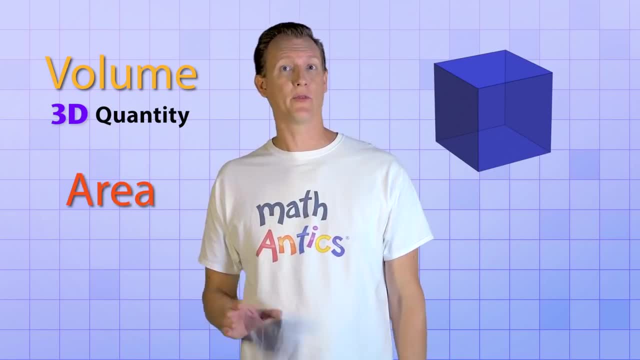 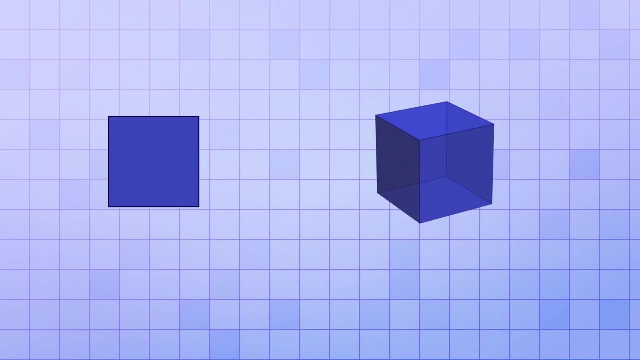 But since we've also talked a lot about area in this video, I want to point out that 3D objects also have a type of area that you don't want to confuse with volume. You might remember from our previous videos that 2D shapes have both a 2D quantity called area. 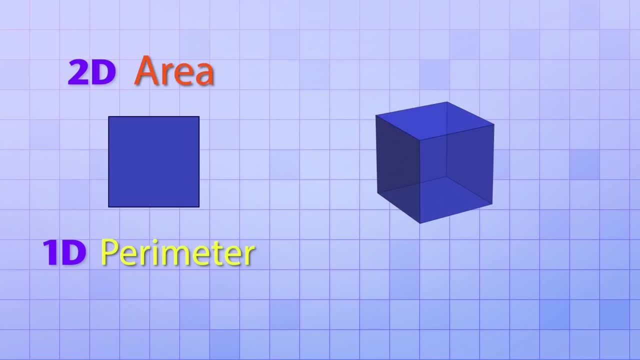 and a 1D quantity called perimeter. Well, in a similar way, 3D objects have both a 3D quantity called volume and a 2D quantity called surface area. Surface area is a lot like it sounds. It's the area of the object's outer surface or shell. 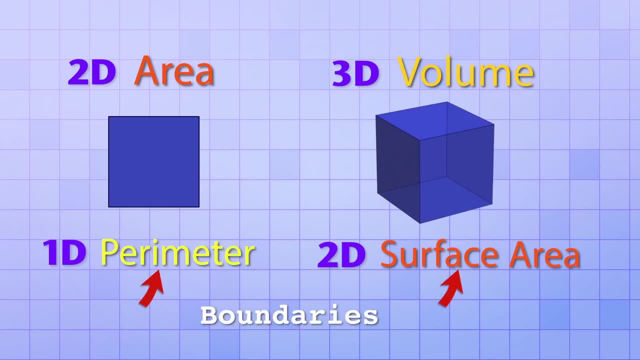 Perimeter and surface area are both outer boundaries of geometric shapes. Perimeter is the one-dimensional outer boundary of a two-dimensional shape and surface area is the two-dimensional outer boundary of a three-dimensional shape. And to help you see the difference between surface area and volume, 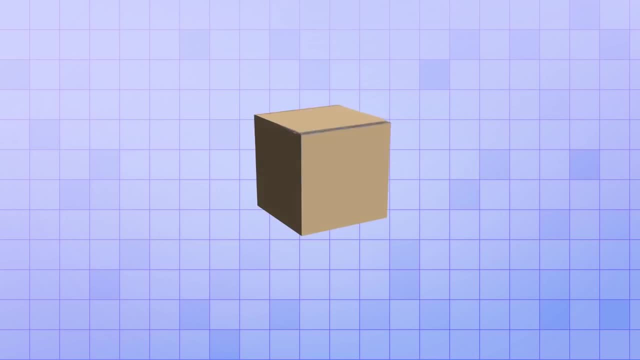 imagine that you have a perfectly thin box filled with ice. If you unfold the box, you can see the 2D area that surrounds the volume, while the volume itself is the amount of 3D space occupied by the ice inside the box. 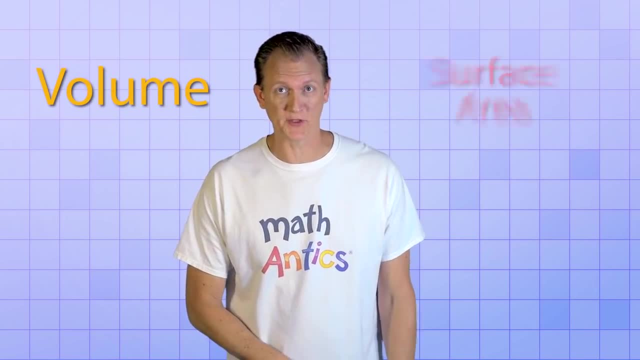 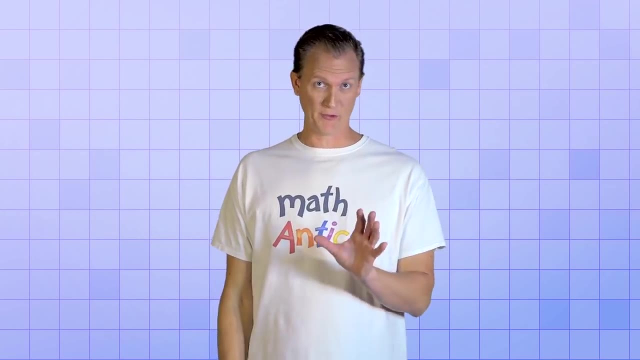 Alright. so now that you understand what volume is and you won't confuse it with surface area, we're going to spend the rest of the video learning how to calculate the volumes of some basic geometric shapes. But before we do that, I want to quickly mention something important about terminology. 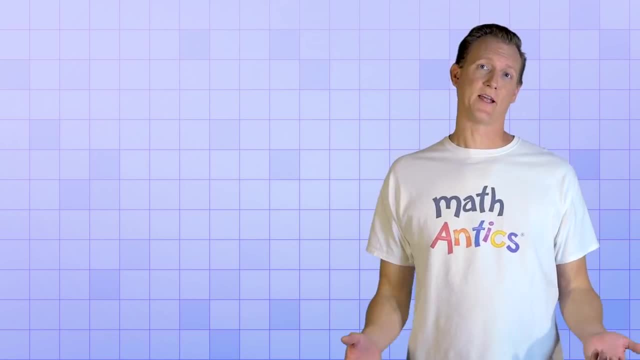 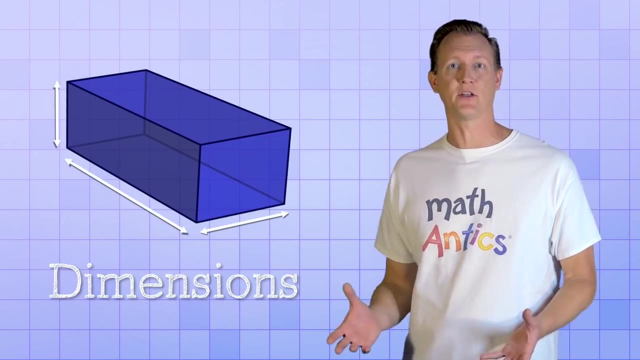 or the words we use to describe things in math. Most of the time, people agree on what to call things in math, but not always. That's especially true when it comes to the words that we use to describe the dimensions of geometric objects. 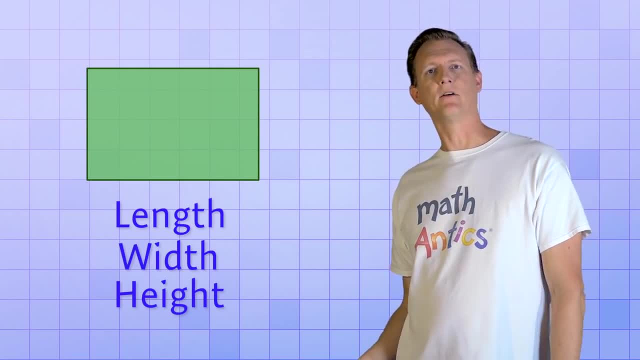 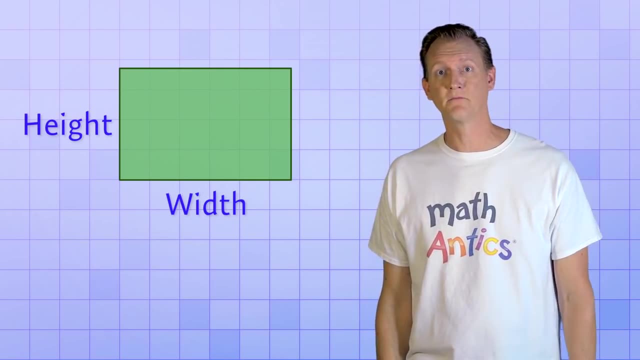 Take the words length, width and height, for example. If I have a rectangle, I could name its two dimensions, length and width, like we did in the area video, But I could also name them width and height if I wanted to. The actual names of the dimensions really aren't important. 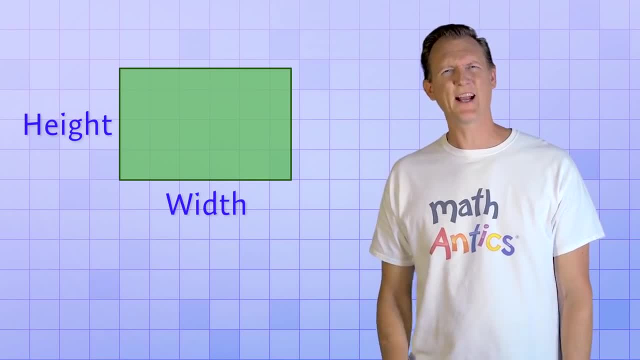 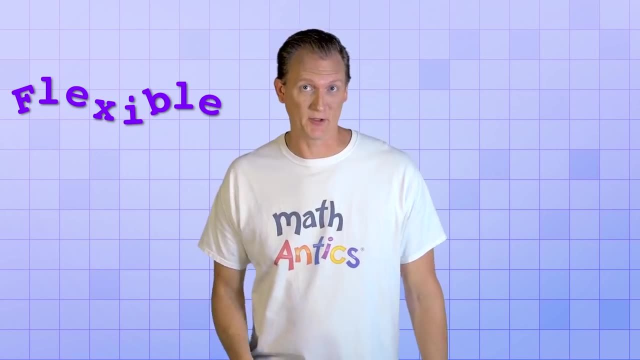 But I could also name them width and height if I wanted to. The actual names of the dimensions really aren't important, so different teachers might use different names. The important thing is to be flexible and realize that the math concepts are the same, even if different words are used to explain them. 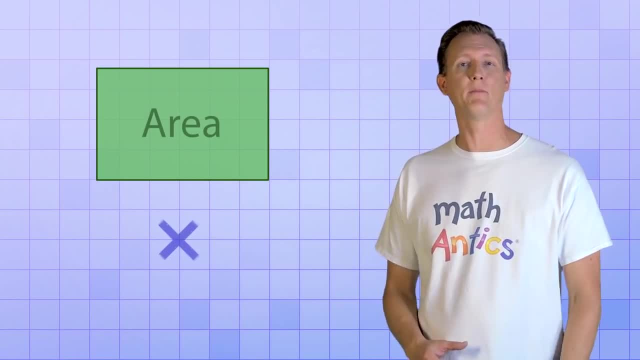 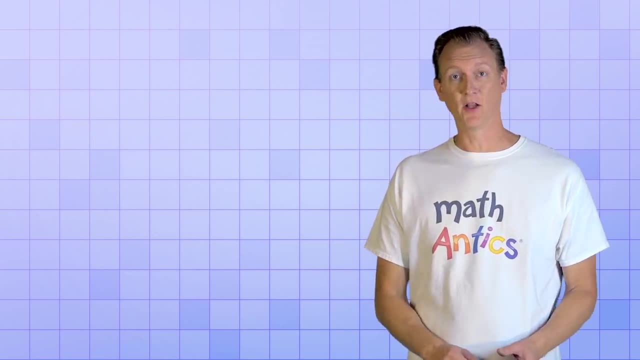 For example, the area of a rectangle is always found by multiplying its two side dimensions together, no matter what they're called. Okay, back to calculating volumes. A lot of 3D shapes can be formed by taking a 2D shape and then extending it along the third dimension. 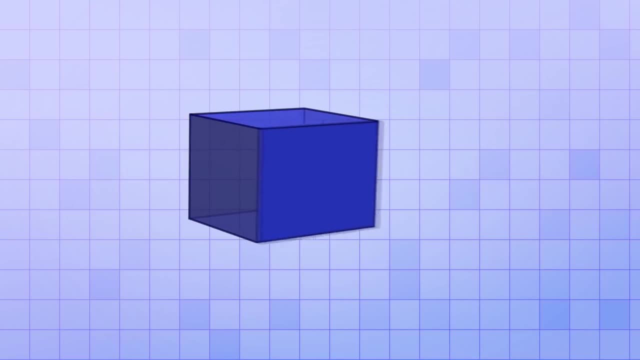 For example, if you start with a rectangle and then extend it along the third dimension, you get a 3D shape called a rectangular prism. If you start with a triangle and then extend it along the third dimension, you get a 3D shape called a triangular prism. 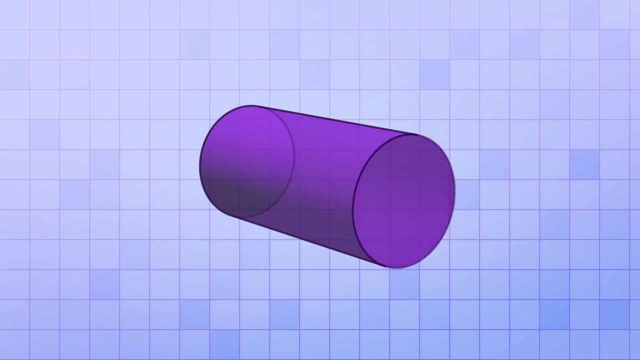 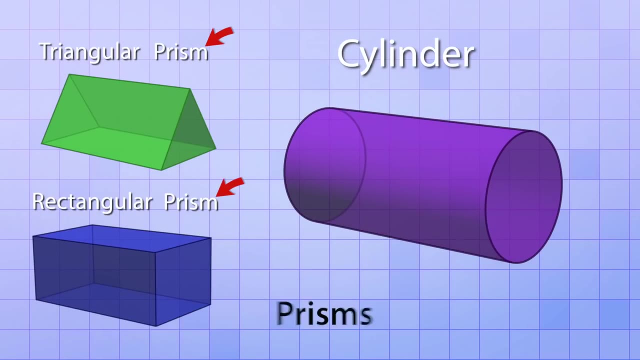 And if you start with a circle and extend it along the third dimension, you get a 3D shape called a cylinder. From the others you might have thought that it should be called a circular prism, But technically prisms are shapes that are formed by extending a polygon. 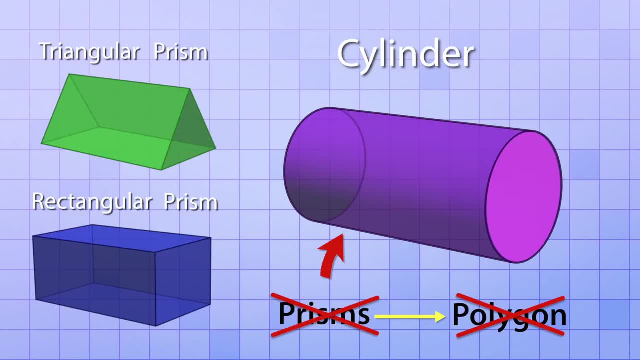 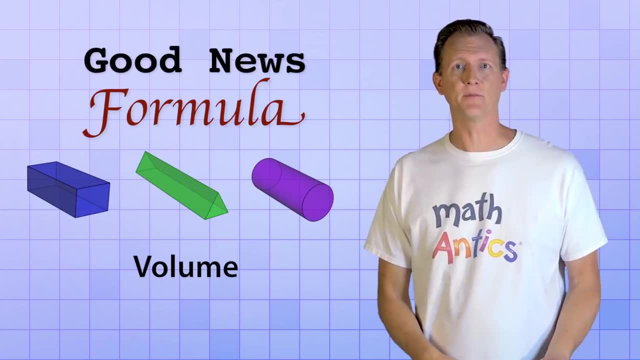 And since a circle is not a polygon, the resulting shape is not called a prism. Okay, so the good news is that there's a general formula for calculating the volume of these types of 3D shapes. All you have to do is find the area of the original 2D shape that got extended. 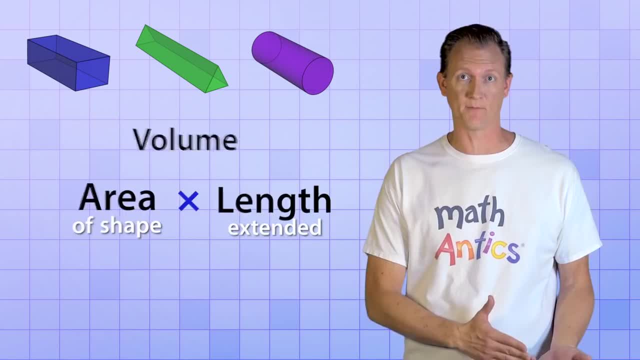 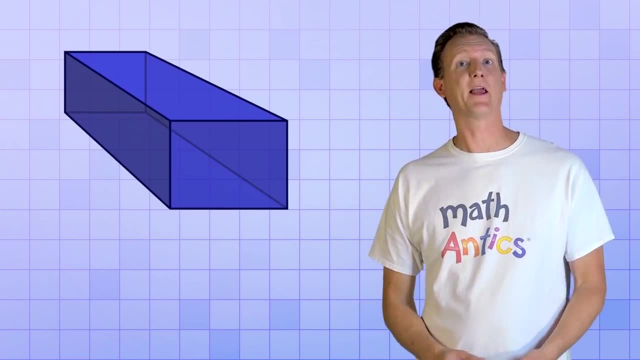 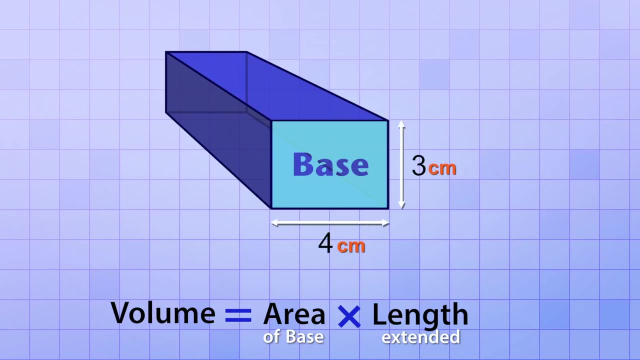 and then multiply that by the length or the distance that it was extended. Usually that original shape is called the base of the object. So let's start with this rectangular prism and calculate its volume. The base is the original rectangle and its dimensions are 4 cm by 3 cm. 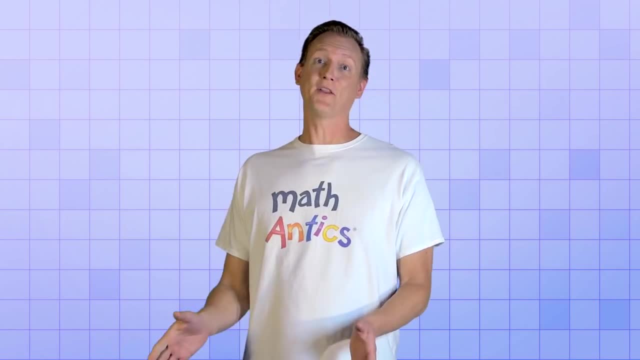 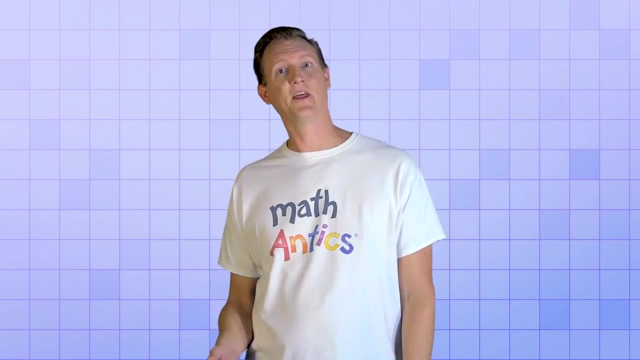 so different teachers might use different names. The important thing is to be flexible and realize that the math concepts are the same, even if different words are used to explain them. For example, the area of a rectangle is always found by multiplying its two side dimensions together. 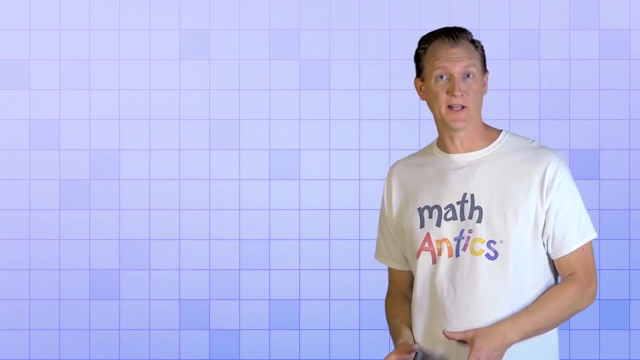 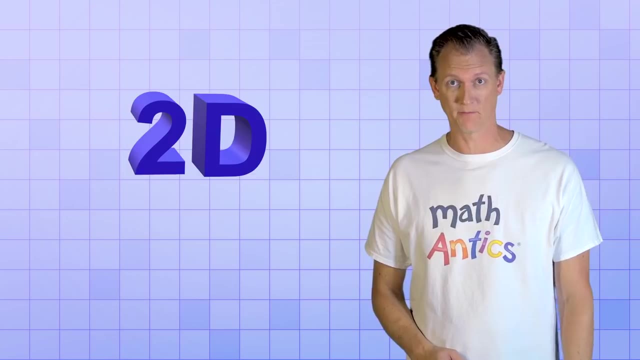 no matter what they're called. Okay, back to calculating volumes. A lot of 3D shapes can be formed by taking a 2D shape and then extending it along the third dimension. For example, if you start with a rectangle and then extend it along the third dimension. 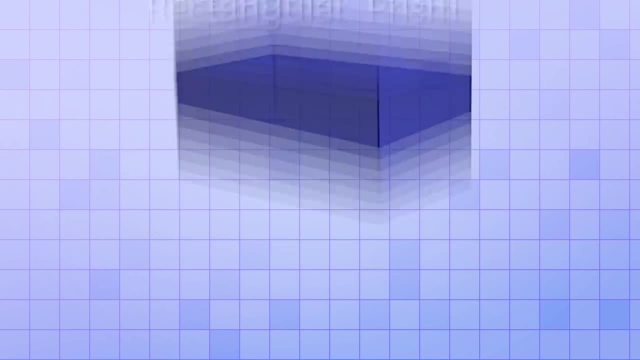 you get a 3D shape called a Rectangular Prism. If you start with a triangle and then extend it along the third dimension, you get a 3D shape called a Triangular Prism. And if you start with a circle and extend it along the third dimension, 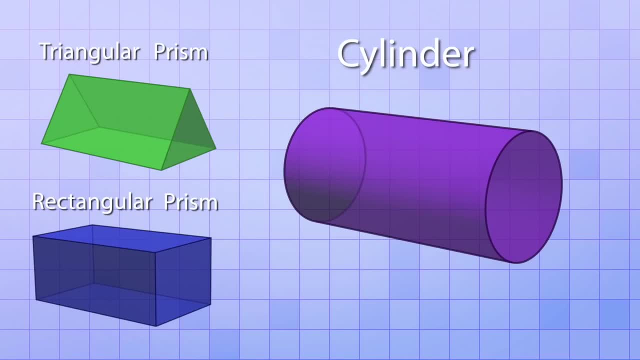 you get a 3D shape called a Cylinder. From the others you might have thought that it should be called a Circular Prism, But technically, prisms are shapes that are formed by extending a polygon, And since a circle is not a polygon, the resulting shape is not called a prism. 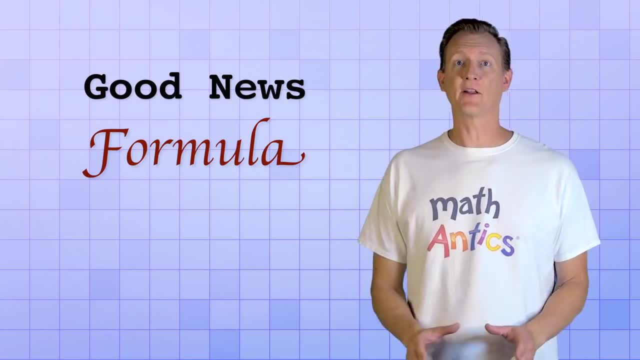 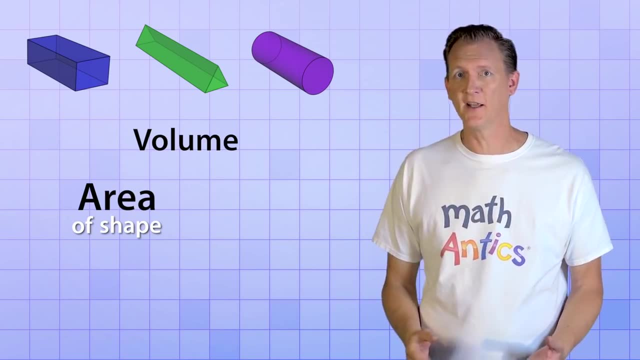 Okay, so the good news is that there's a general formula for calculating the volume of these types of 3D shapes. All you have to do is find the area of the original 2D shape that got extended and then multiply that by the length or distance that it was extended. 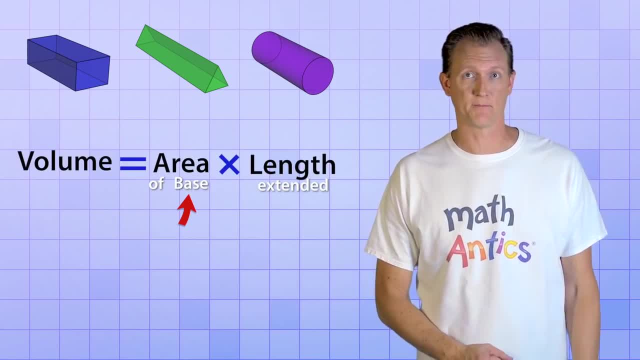 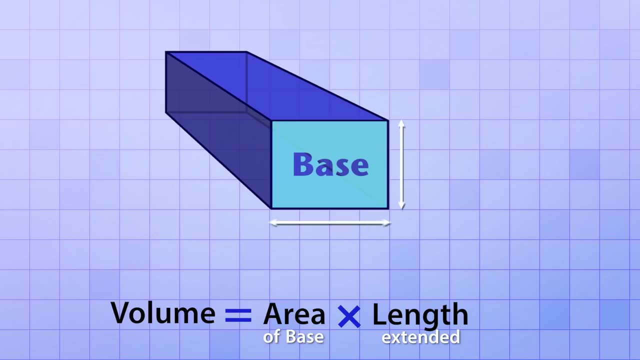 Usually that original shape is called the base of the object. So let's start with this Rectangular Prism and calculate its volume. The base is the original rectangle and its dimensions are 4 centimeters by 3 centimeters. So to find the area of that base, we need to remember how to calculate the area of a rectangle. 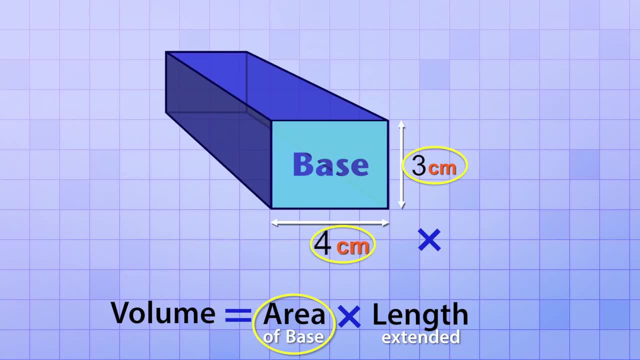 To do that, we just multiply the two side dimensions together. 4 centimeters times 3 centimeters gives us 12 centimeters squared. Now to find the volume, we just need to multiply that area by the length that the base was extended. 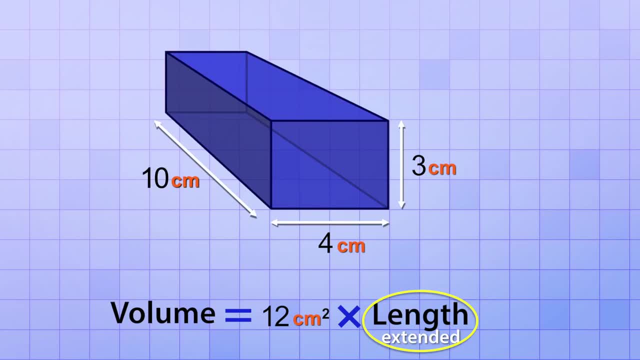 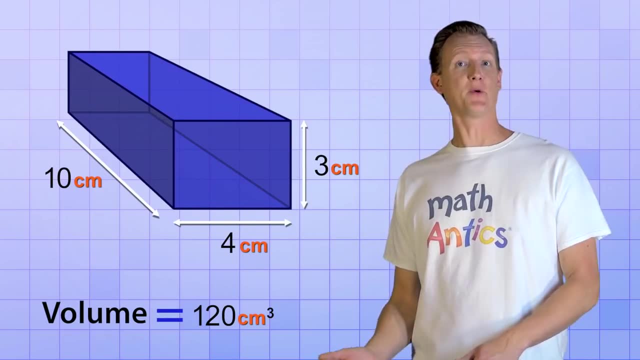 Our diagram tells us that distance is 10 centimeters. So if we multiply 12 centimeters squared by 10 centimeters, we get 120 centimeters cubed. So this Rectangular Prism has a volume of 120 cubic centimeters. 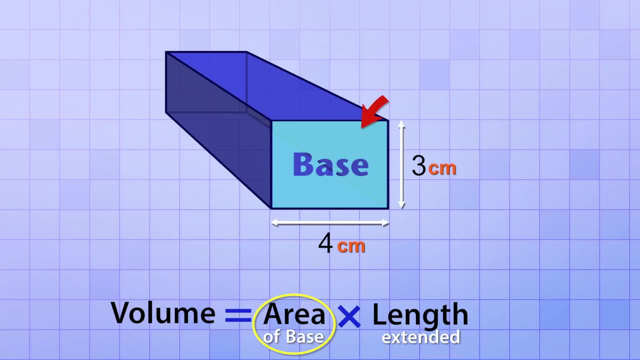 So to find the area of that base, we need to remember how to calculate the area of a rectangle. To do that, we just multiply the two side dimensions together. 4 cm times 3 cm gives us 12 cm squared as the area. 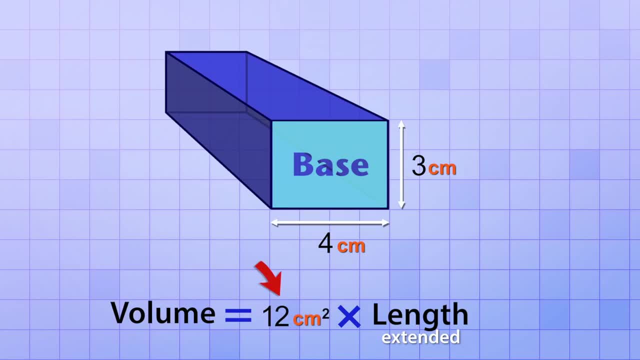 Now to find the volume, we just need to find the area of the original 3D shape. To find the volume, we just need to multiply that area by the length that the base was extended. Our diagram tells us that distance is 10 cm. 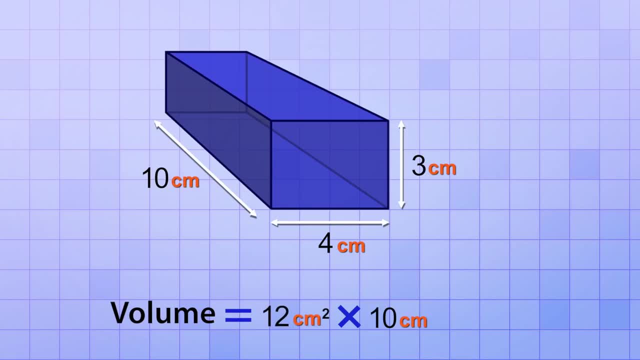 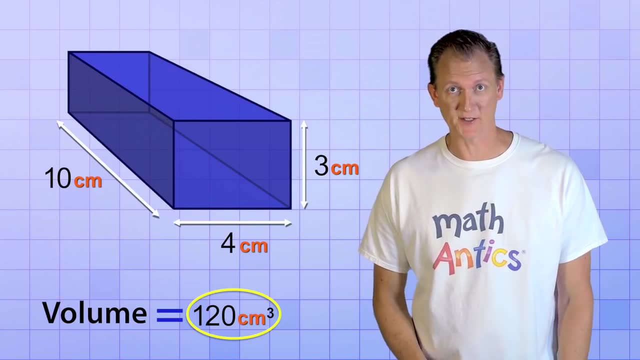 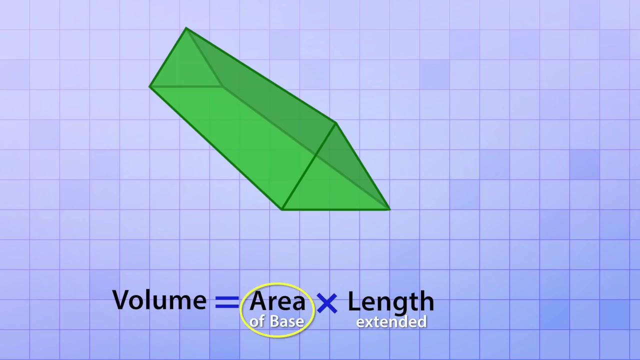 So if we multiply 12 cm squared by 10 cm, we get 120 cm cubed. So this rectangular prism has a volume of 120 cubic centimeters. Okay, let's try to find the volume of the triangular prism. now, Again, the first step is to calculate the area of the base of the prism, which is the triangle. 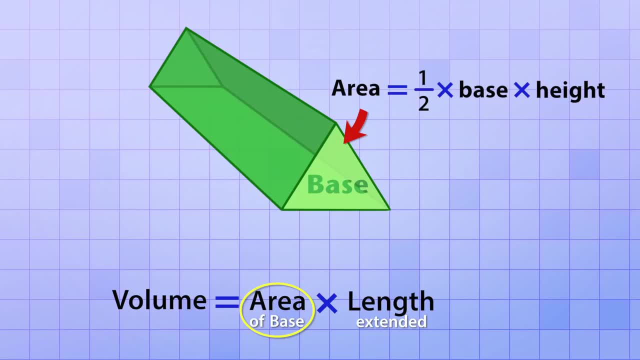 The formula for finding the area of a triangle is one half of the triangle's base times its height. Be careful not to confuse the base of the triangle with the base of the prism, which is the triangle itself. Our diagram tells us that the base of the triangle is 10 inches and its height is 8 inches. 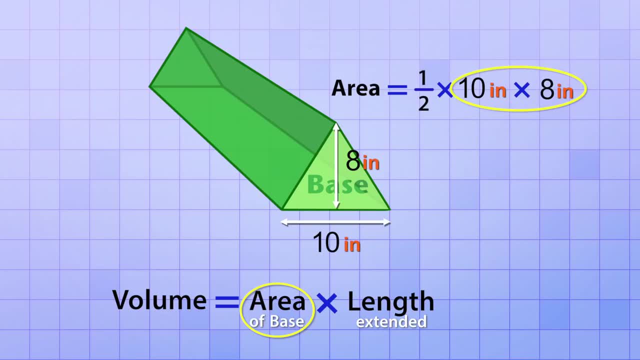 So one half the base times the height would be one half of 10 times 8.. 10 times 8 is 80, and one half of 80 is 40, so the area of the triangle is 40 inches squared. Now all we have to do to find the volume is to find the area of the triangle. 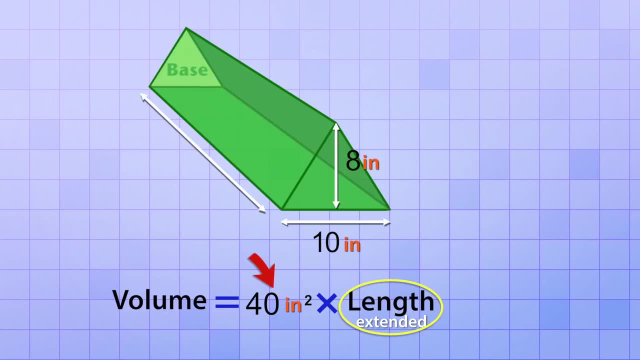 Now all we have to do to find the volume is to multiply that area by the length that it was extended. We're told that the length is 50 inches, so we multiply 40 inches squared by 50 inches and we get 2000 inches cubed. 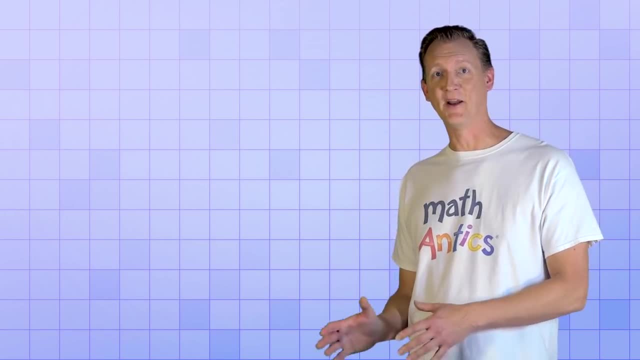 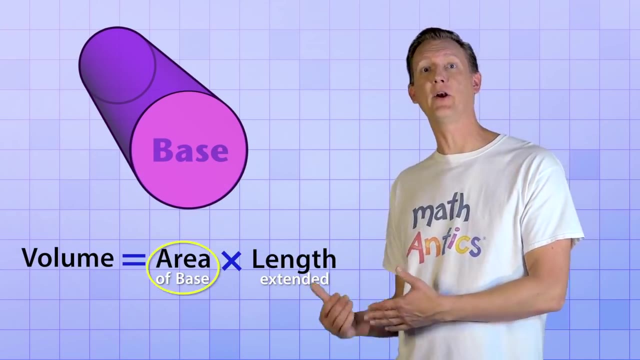 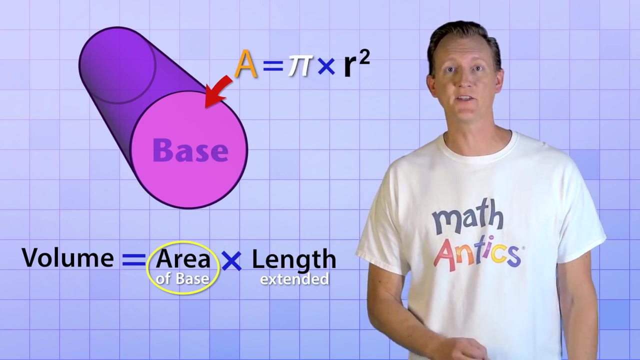 That's the volume of this prism. Alright, are you ready to try finding the volume of the cylinder now? The cylinder is made by extending a circle, so first we need to calculate the area of that circle. As we learned in a previous video, the area of a circle is found by multiplying pi times its radius squared. 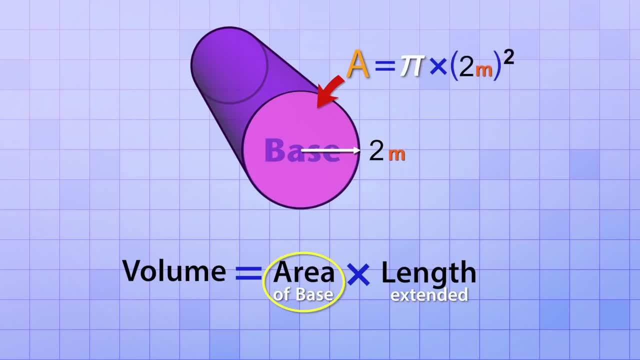 The radius of this circle is the area of the circle. The radius of this circle is the area of the circle. This circle is 2 meters. so if we square that, we get 4 meters squared. Then we multiply by pi, which is approximately 3.14, and we get 12.56 meters squared. 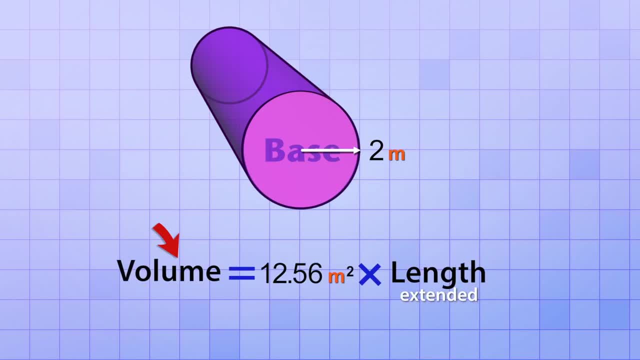 Now that we know the area of the circle, to find the volume of the cylinder we just multiply that area by the length that the circle was extended, which happens to be 10 meters. 10 meters times 12.56 meters squared gives us 125.6 meters cubed, so the volume of this cylinder. 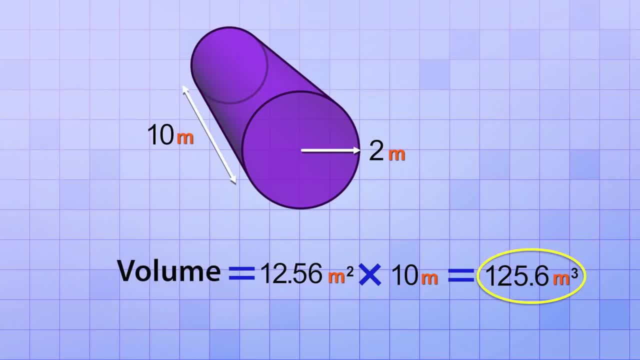 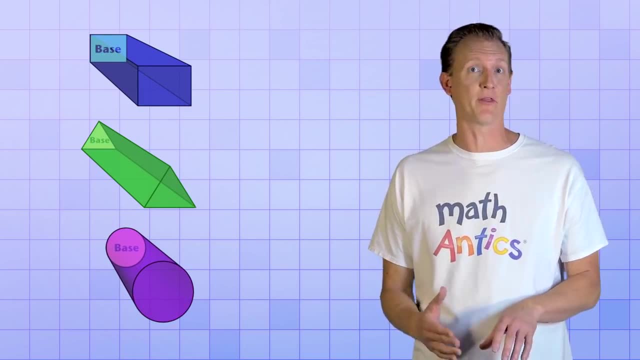 is 125.6 cubic meters. So do you see how to find the volume of 3D shapes like these? Shapes that are made by taking a 2D shape and then extending it along a third axis? You just find the area of that shape and then you multiply it by the length that it was extended. 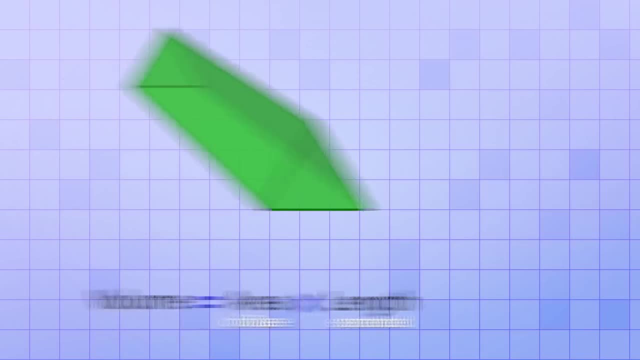 Okay, let's try to find the volume of the Triangular Prism. now Again, the first step is to calculate the area of the base of the prism, Which is the triangle. The formula for finding the area of a triangle is one half of the triangle's base times its height. 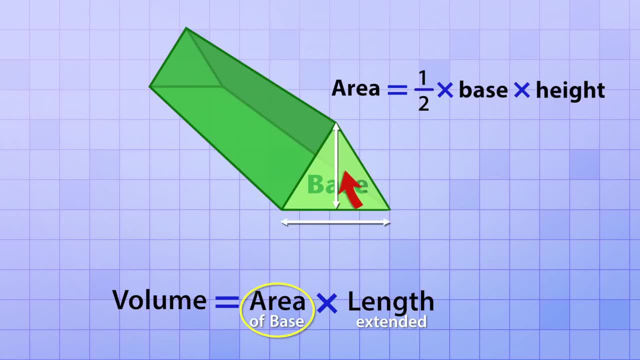 Be careful not to confuse the base of the triangle with the base of the prism, which is the triangle itself. Our diagram tells us that the base of the triangle is 10 inches and its height is 8 inches. So one half the base times the height would be one half of 10 times 8.. 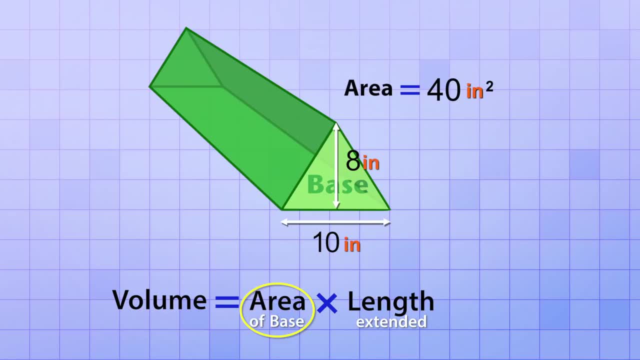 10 times 8 is 80. And one half of 80 is 40. So the area of the triangle is 40 inches squared. Now all we have to do to find the area of the triangle is to find the area of the prism. 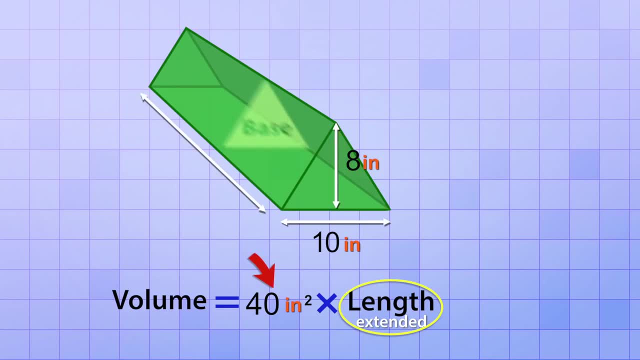 All we have to do to find the volume is to multiply that area by the length that it was extended. We're told that the length is 50 inches, so we multiply 40 inches squared by 50 inches and we get 2000 inches cubed. 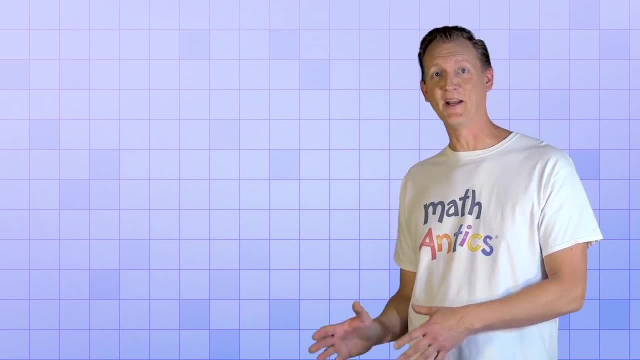 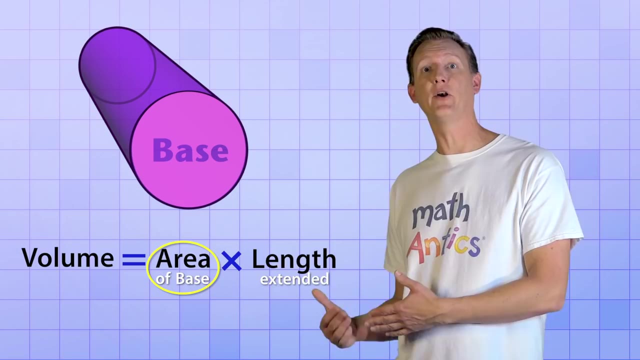 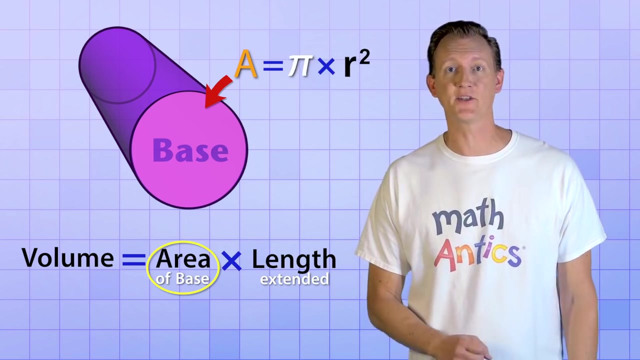 That's the volume of this prism. Alright, are you ready to try finding the volume of the cylinder now? The cylinder is made by extending a circle, so first we need to calculate the area of that circle. As we learned in a previous video, the area of a circle is found by multiplying pi times its radius squared. 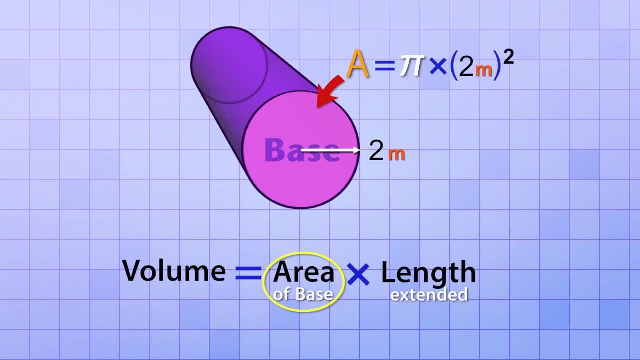 The radius of this circle is 2 meters. So if we square that, we get 4 meters squared. Then we multiply by pi, which is approximately 3.14, and we get 12.56 meters squared. Now that we know the area of the circle, to find the volume of the cylinder we just multiply that area by the length that the circle was extended. 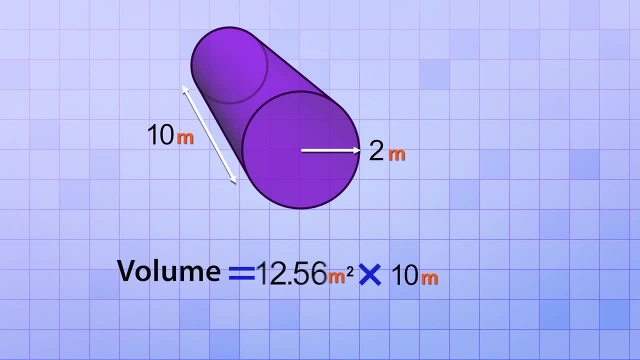 which happens to be 10 meters. 10 meters times 12.56 meters squared gives us 125.6 meters cubed, So the volume of this cylinder is 125.6 cubic meters. So do you see how to find the volume of 3D shapes like these? 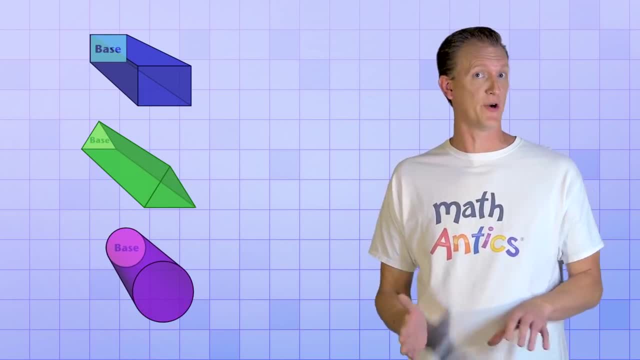 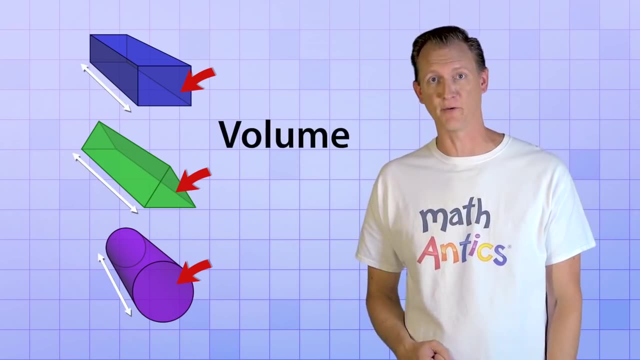 Shapes that are made by taking a 2D shape and then extending it along a third axis. You just find the area of that shape and then you multiply it by the length that it was extended and that gives you the volume, And it works for any 2D shape. 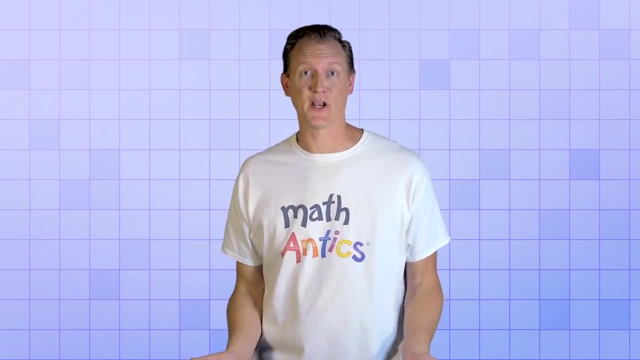 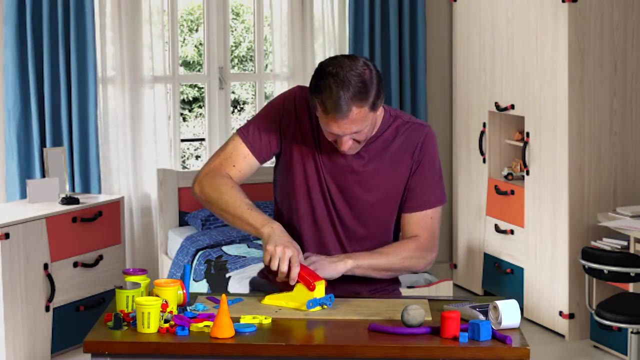 and that gives you the volume, And it works for any 2D shape. It works for trapezoids or pentagons or diamonds, or stars or hearts… Alright, meh, Now that I know how to do this, I'm going to go ahead and do it. 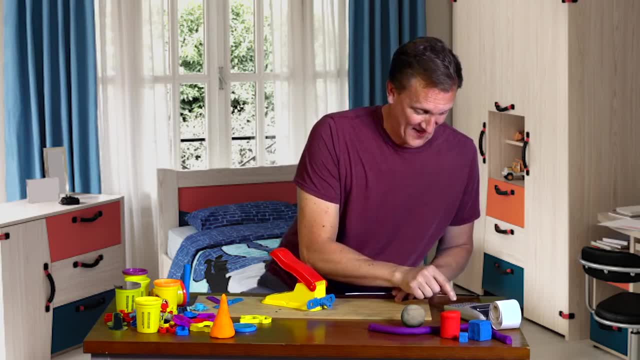 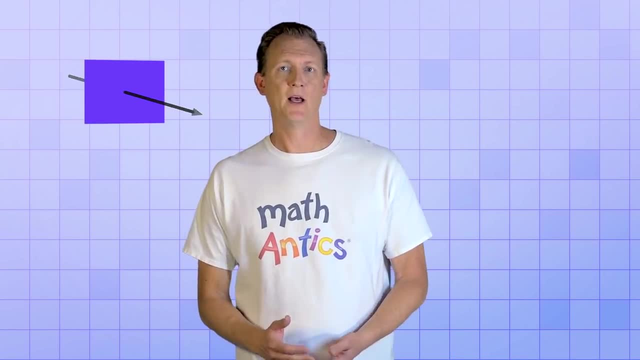 Now that I know how to accurately calculate volumes, playtime is way more fun. Of course, not all 3D shapes are made by extending a 2D shape along a third dimension. Some are made by rotating a shape around an axis, like the sphere we saw earlier in the video. 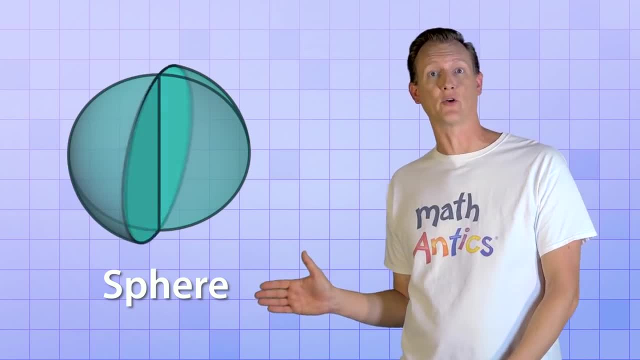 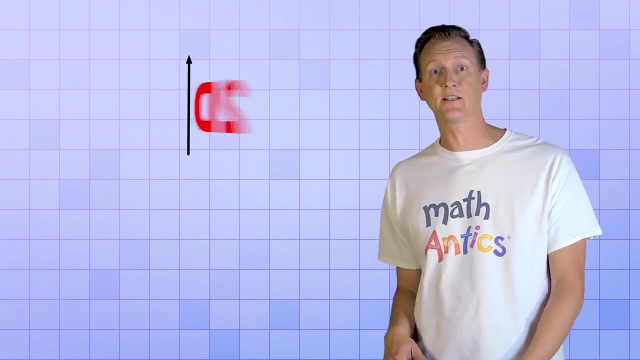 for instance, One way to form a sphere is to rotate a 2D circle around one of its diameter lines, And another common 3D shape that can be formed by rotating a 2D shape around an axis is a cone. A cone can be formed by rotating a right triangle. 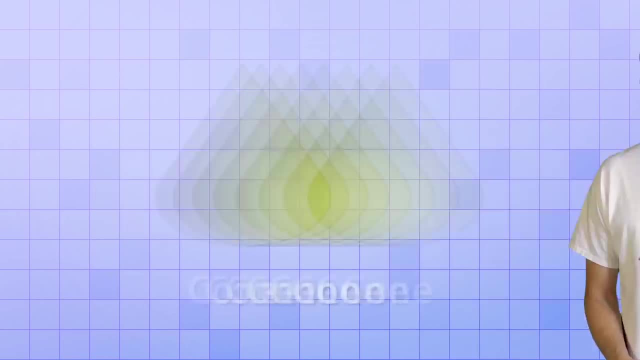 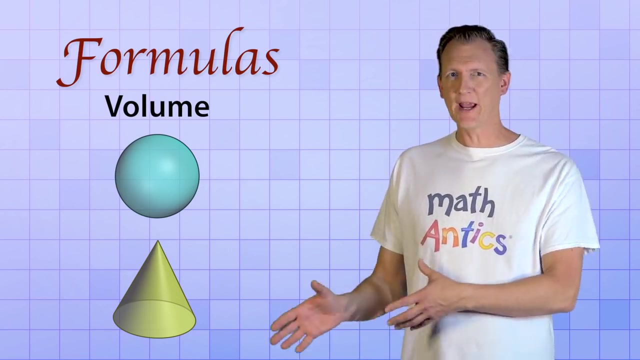 around one of its two perpendicular edges. Since the formulas for finding the volumes of spheres and cones are more complicated to explain, we don't have time to learn how we arrive at them in this video. So for now it's best if you just memorize the formulas so you can use them on tests if you need to. 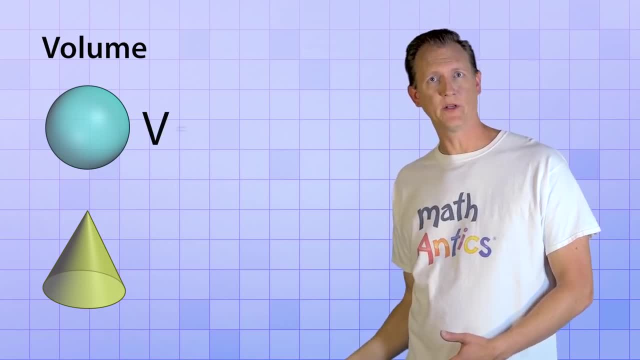 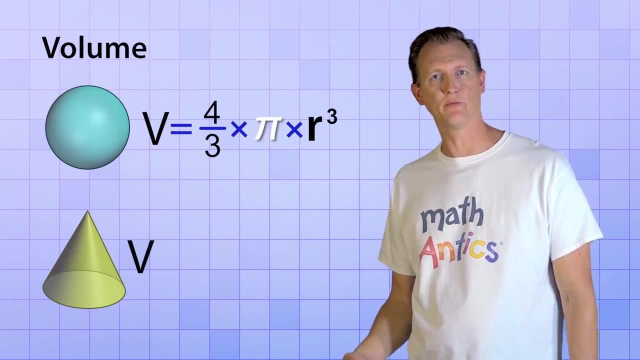 To find the volume of a sphere, you use the formula volume equals four thirds times pi times radius cubed. And to find the volume of a cone, you use the formula volume equals one third times height times pi times square. Let's try one example of each before we wrap up. 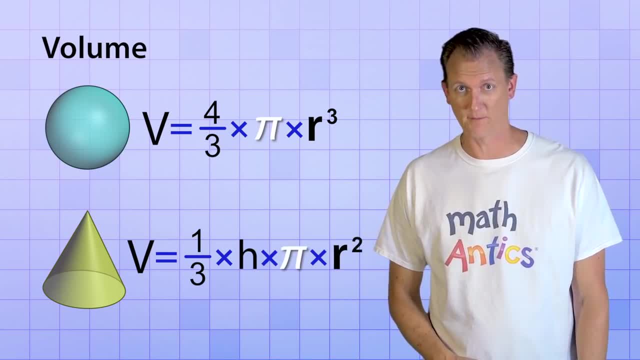 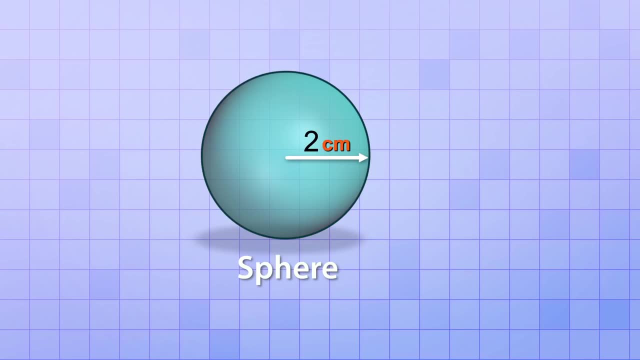 Here's a sphere with a radius of two centimeters. Fortunately, that's the only dimension. we need to find its volume. Our formula says that the volume of a sphere is equal to four thirds times pi times radius cubed. Cubing the radius means multiplying it by itself three times. 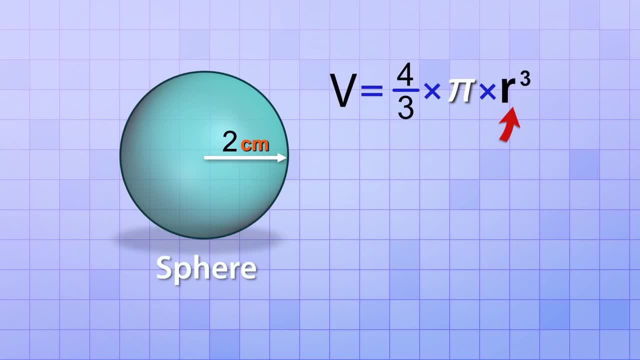 So we take two centimeters times two centimeters times two centimeters, which equals eight centimeters cubed. Next we'll multiply the radius of the sphere by the radius of the cone. So we have two centimeters times two centimeters times two centimeters. 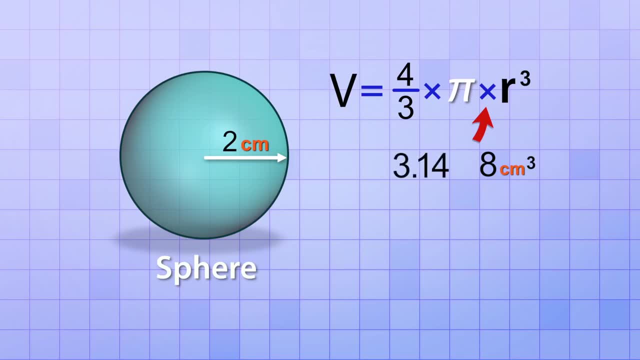 so we'll multiply that by our approximation for pi. 3.14 times 8 is 25.12.. And last, we multiply that by four thirds, which is the same as multiplying by four, then dividing by three, which gives us a volume of 33.49 centimeters cubed. 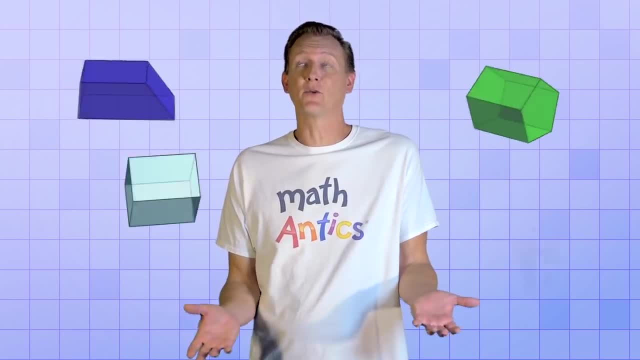 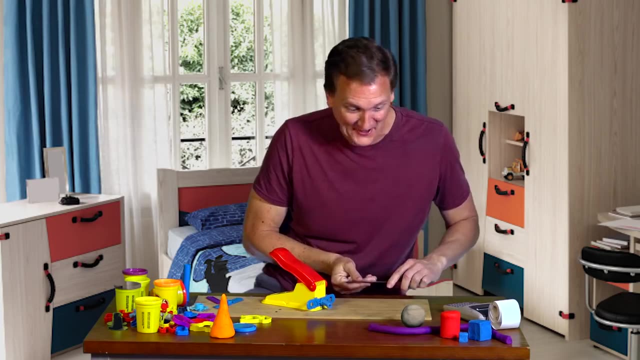 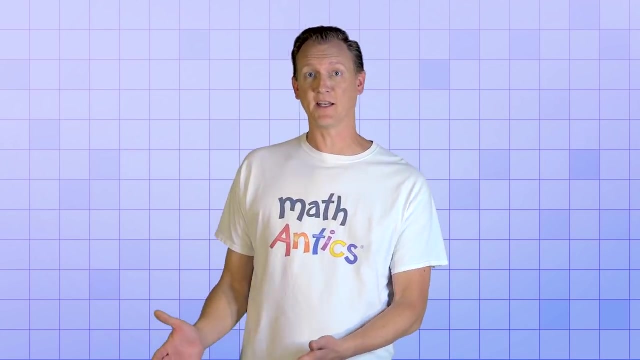 It works for trapezoids or pentagons or diamonds or stars or hearts… Alright, man, Now that I know how to accurately calculate volumes, playtime is way more fun. Of course, not all 3D shapes are made by extending a 2D shape along a third dimension. 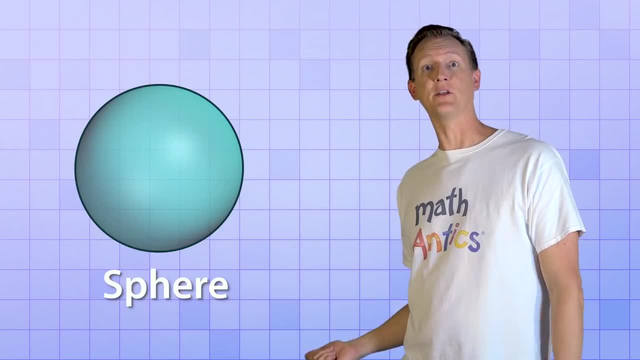 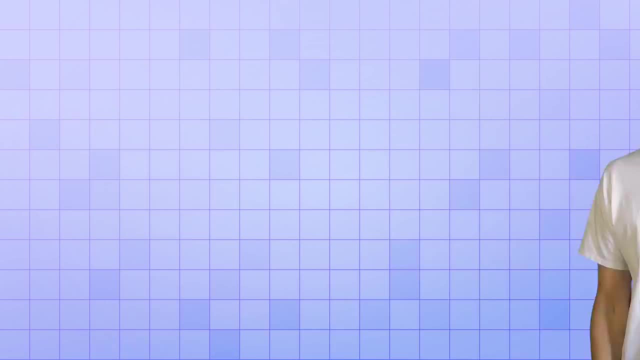 Some are made by rotating a shape around an axis, like the sphere we saw earlier in the video. for instance, One way to form a sphere is to rotate a 2D circle around one of its diameter lines, And another common 3D shape that can be formed by rotating a 2D shape around an axis is a cone. 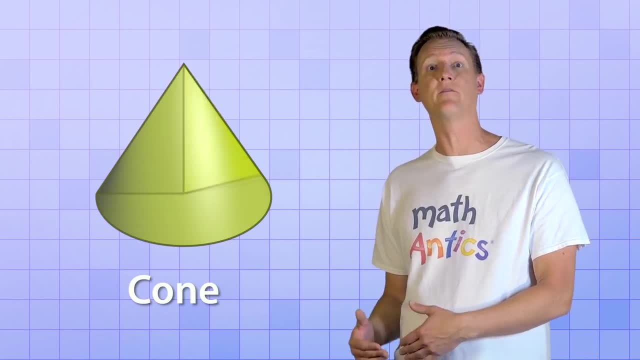 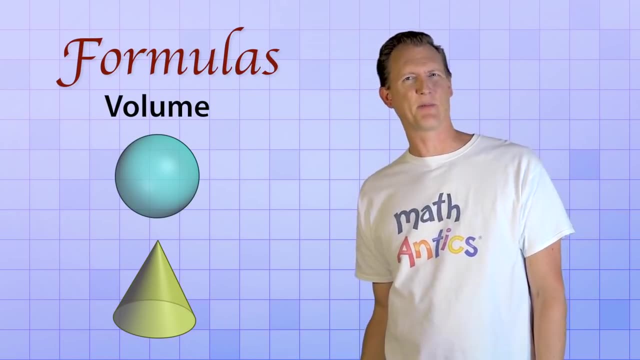 A cone can be formed by rotating a right triangle around one of its two perpendicular edges. Since the formulas for finding the volumes of spheres and cones are more complicated to explain, we don't have time to learn how we arrive at them in this video. 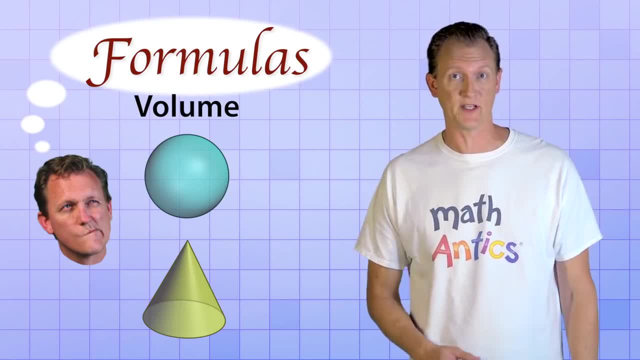 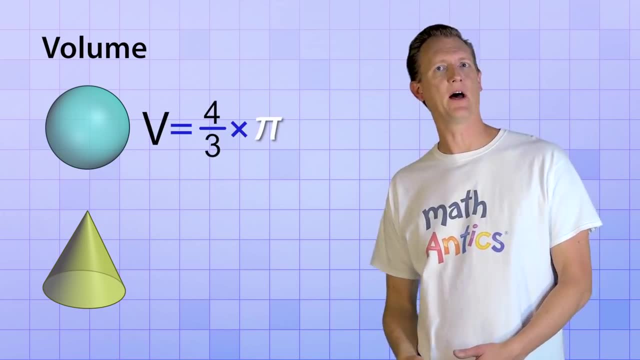 So for now it's best if you just memorize the formulas so you can use them on tests if you need to. To find the volume of a sphere, you use the formula volume equals four thirds times pi, times radius cubed. And to find the volume of a cone, you use the formula. 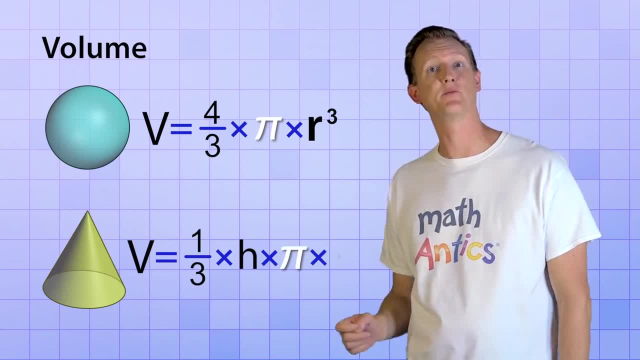 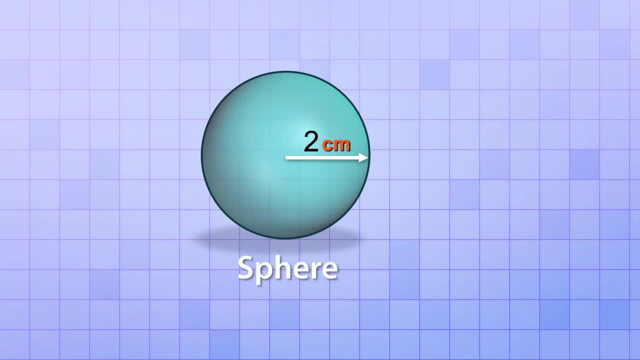 volume equals 1 third times height times pi times pi times radius squared. Let's try one example of each before we wrap up. Here's a sphere with a radius of 2 cm. Fortunately, that's the only dimension. we need to find its volume. 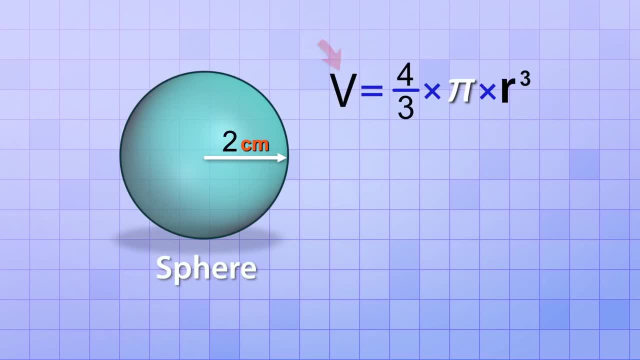 Our formula says that the volume of a sphere is equal to 4 thirds times pi times radius cubed. Cubing the radius means multiplying it by itself 3 times. So we take 2 cm times 2 cm times 2 cm, which equals 8 cm cubed. 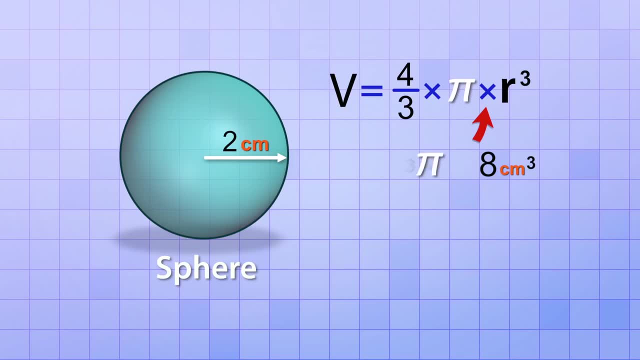 Next, we'll multiply that by our approximation for pi. 3.14 times 8 is 25.12.. And last, we multiply that by 4 thirds, which is the same as multiplying by 4, then dividing by 3,. 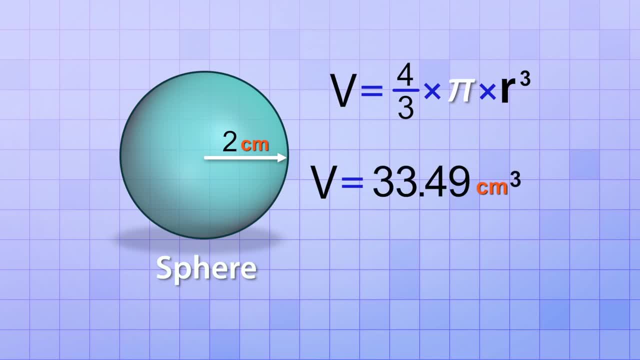 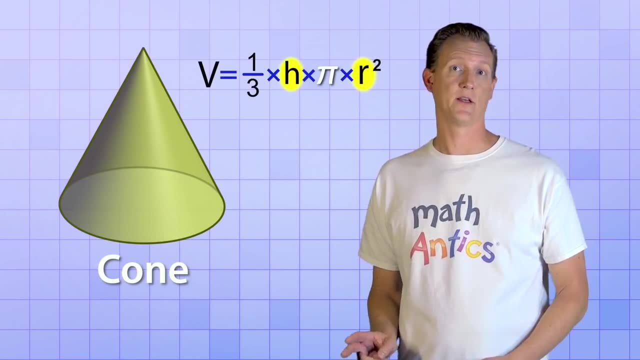 which gives us a volume of 33.49 cm cubed. Now let's try a cone. To use our formula. to find the volume of a cone we need to know two things: The radius of the circle that forms the base of the cone.